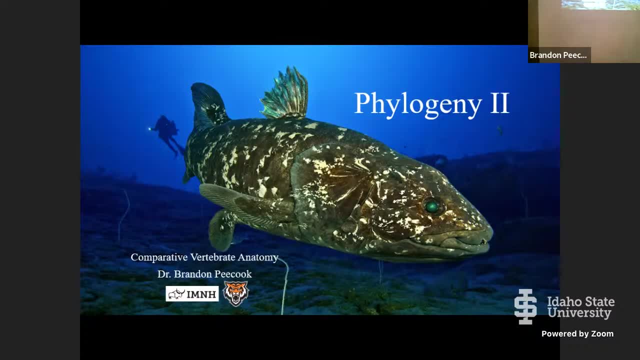 ability to look. So on the Moodle page, if you haven't seen it yet, there's a YouTube link And as we go through the course, lectures will be put up on YouTube for you to look at, kind of like in review. I would encourage you to not rely on them via your participation, But anyway. 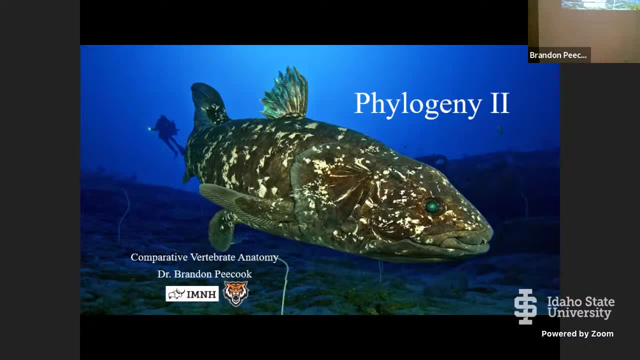 we're going to pick up where we left off with phylogeny and evolutionary trees. People know this fish, Yeah, coelacanth. So one of these fishes that we call a lobe fin fish, a fish that's got a lot of muscles and bones right here in the base of its fin, that, if you don't know what a 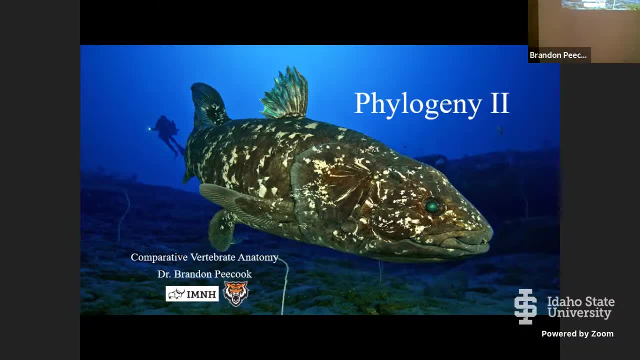 coelacanth is obviously. that's completely fine. We're going to talk about it later, But after the king cobra thing I kind of liked that coelacanths were like a topic a little bit last time And so 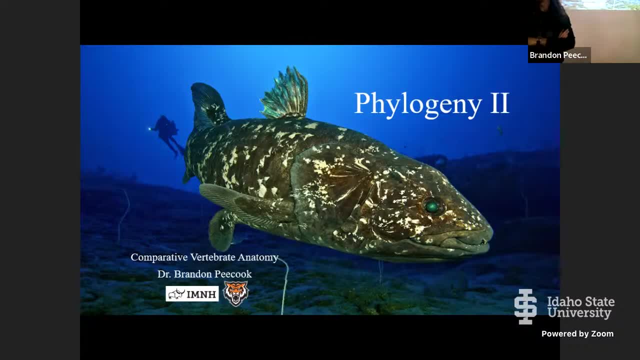 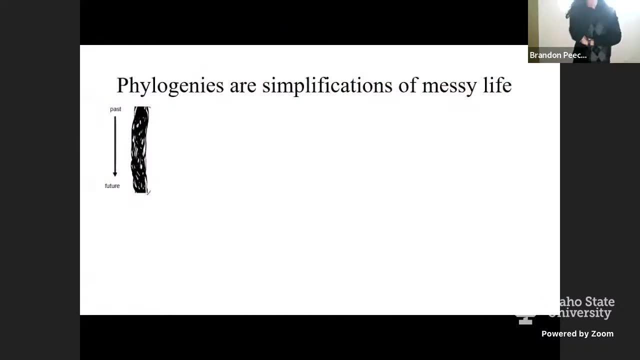 I think maybe that's how I'll choose our little cover slides, because who cares what's on the cover slide? Just me And maybe you guys. So phylogeny, And so where we left off, you guys have learned a little bit. 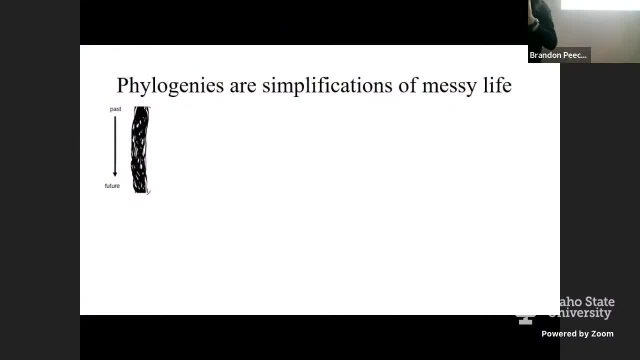 of if you hadn't before, or at least you were refreshed a little bit of like reading phylogeny. So the cow and the trout and the coelacanth, What do these different lines mean? It's all about the way the lines connect. These are diagrams that show relationships. They show 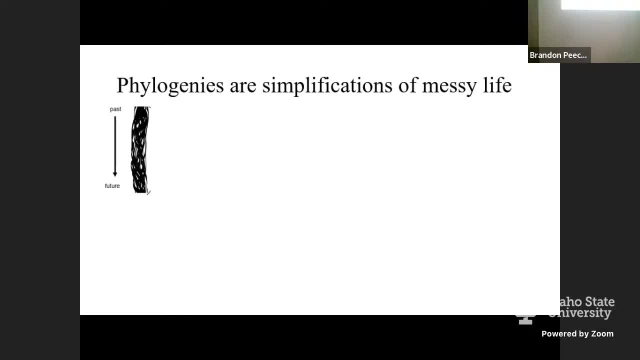 evolution. Evolution is descent with modification. They are tools for us. We are in an applied class. We are not a class that's about phylogenetics. They're our class, So we're going to be using trees to answer questions. Trees are another way to test. 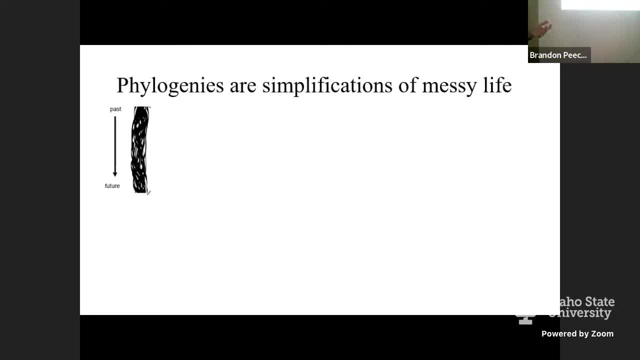 hypotheses that you or any other scientist might have in evolutionary biology, And so something that I want to make really clear to you- and this is something that I think is actually very beautiful- is that phylogenies are these like extremely simple things That trout coelacanth. 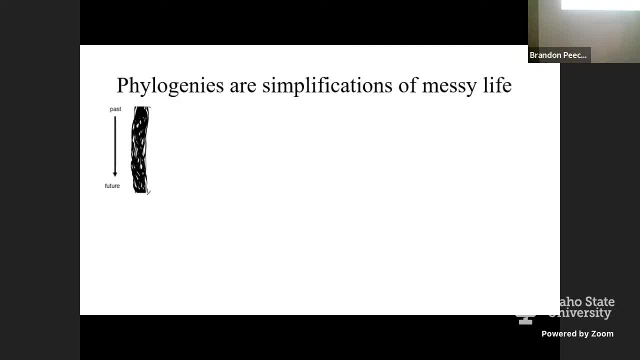 cow from last Thursday where we just had them. like this: three lines to show you something really important about the history of like vertebrate life. That is very useful and very functional, But of course the real thing is so much crazier and more interesting, And so these are some. 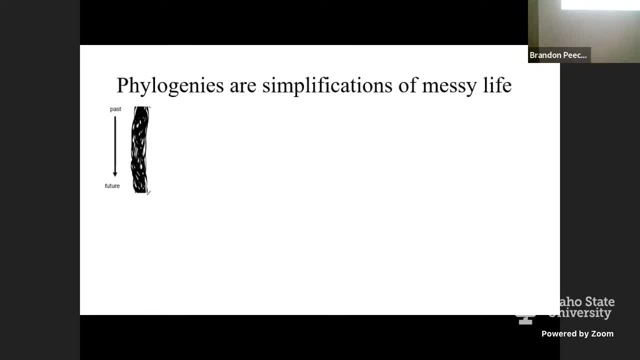 really famous diagrams. They're kind of upside down and backwards and all that because how? maybe we would talk today, But I really want you guys to see them. So you guys know, I think from your intro bio courses and maybe something like ecology or something like that, if they talk about it. 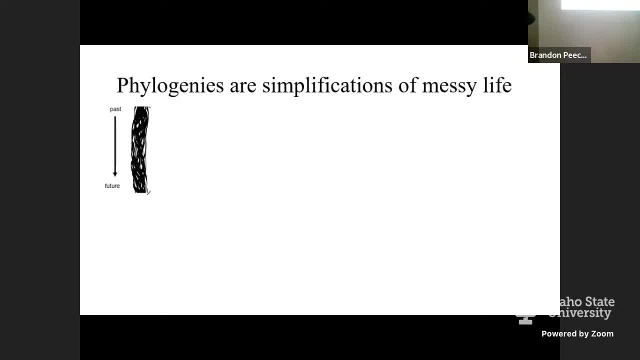 Evolution. yes, it's descent with modification, But, like in the actual moment, what evolution is? it's like changing allele frequencies, right, And populations of breeding organisms, or at least reproducing organisms. So that's what evolution actually is. And so what I like about phylogeny and things like: 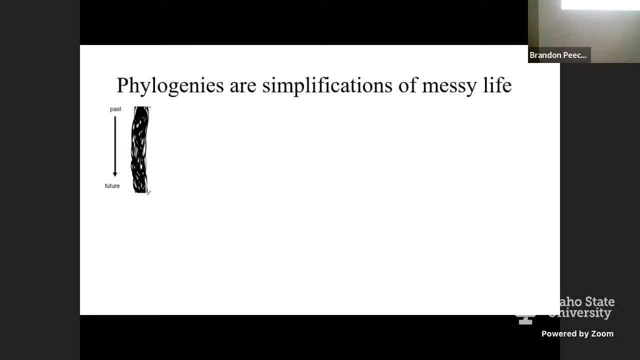 paleontology is that. it's like so far removed, It's like way up there And you're looking at five fossils. There's no population, There's no, you know, capital, P, lowercase p, punnett, square in making something like macroevolution, which is really big. So this is like a really fun. 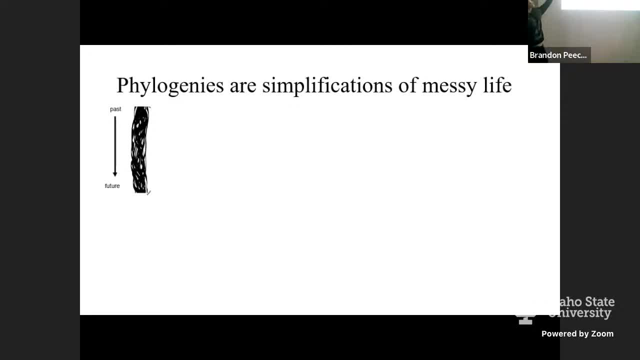 diagram, I think. So past up at the top, future down at the bottom, And so I think in the modern we would turn this upside down. This is like this classic figure I really like. What you're supposed to be seeing there is that if you zoom in, if you were to go like this on the little phylogeny that 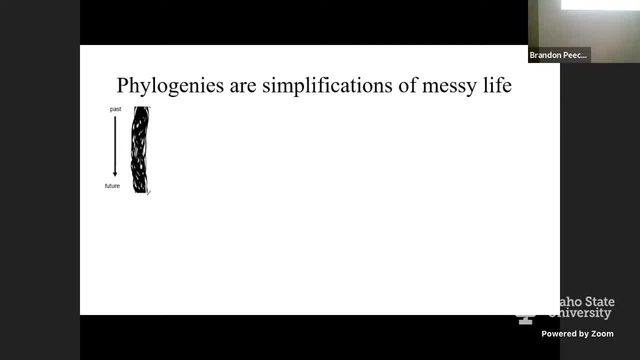 we looked at last week with the cow and the coelacanth and the trout and zoom in on that line in real life leading up to the cow, if you zoomed in far enough, kind of like if you zoomed in on a 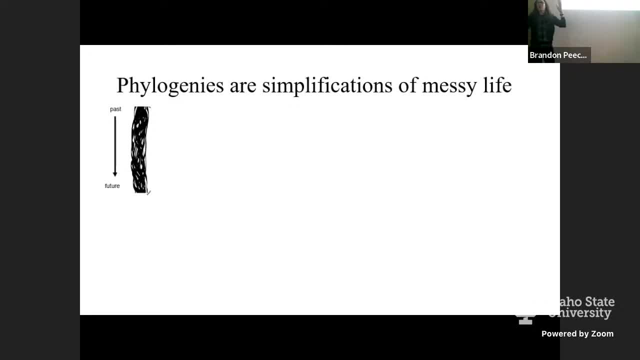 chromosome you get to like, you know, the DNA Those are supposed to represent, like populations in time that are kind of weaving back and through each other. So imagining the line on the phylogeny as not like a monolith leading towards cows, but as like the history of the population. 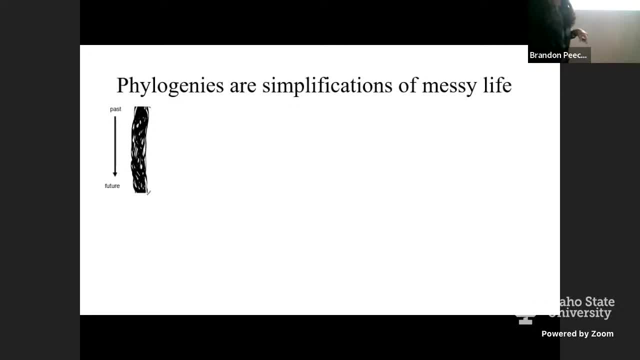 Leading up to where that cow is now. So let me show you another zoom in just to help you see what I'm talking about. That's supposed to be like a zoom in on this, And so maybe in the past there was one ancestral thing, And now maybe down here there's four things that we live with in the 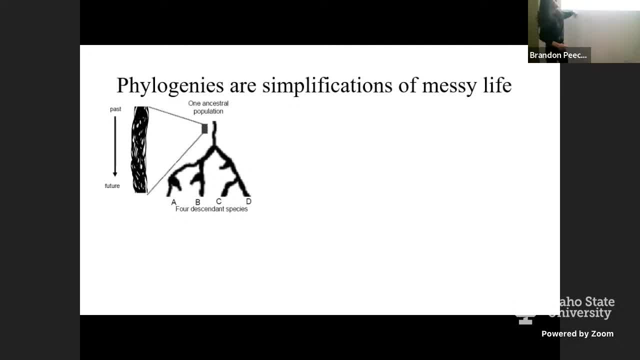 present A, B, C and D. But if we go back and zoom in on any of those lines we can see that in real life the way the world really works is like there's all kinds of populations of whatever's happening there before any kind of split happens, And then you can see there's other splits that 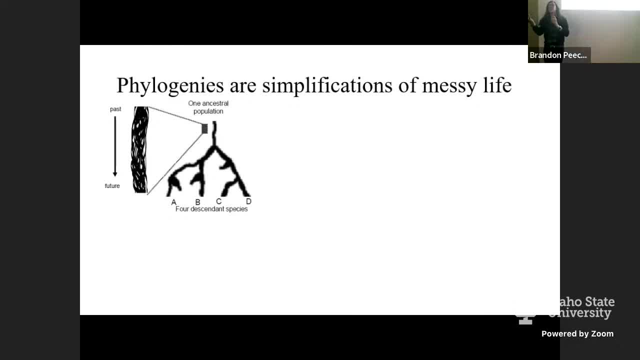 happen later. There's other splits that happen later, And then you can see there's other splits that happen, but then the descendants of that split aren't alive anymore, They're extinct. They don't exist. That population went away. Maybe that was a new species that went away, And so the real 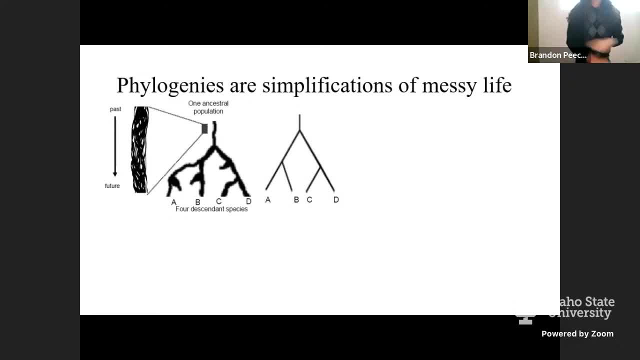 world looks something like that: You and I in a biology classroom are always going to be talking like this, And I know this might seem a little bit like wooey-wowey, but I just think it's really important that we're going to be doing this kind of drawing all the time. But as biologists, I want. 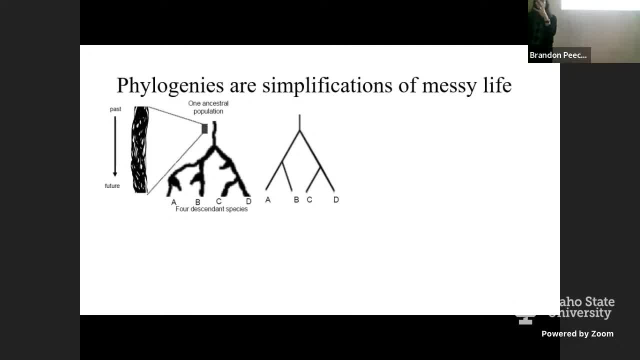 you guys to keep in mind that the real world is something like that. We're only ever kind of approximating, And so phylogenies are simplifications and they're very useful, but they're not supposed to be these standalone things that are absolute. This is a really cool example of phylogeny that I think. 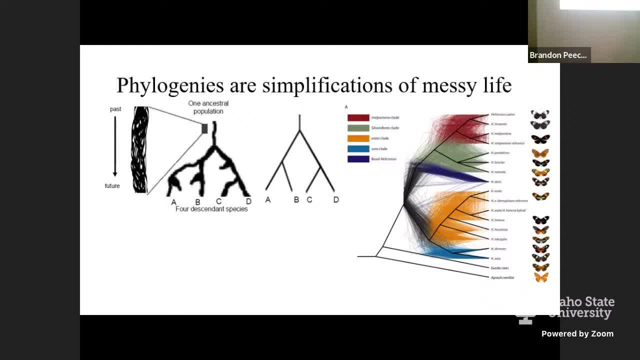 you know, if this was a genetics class or if we were doing phylogeny, for, like our actual point of our class, we probably spent a lot of time on this. I just think it's cool for you guys to see. You can see the black lines here which represent the actual inferred phylogeny that humans are very 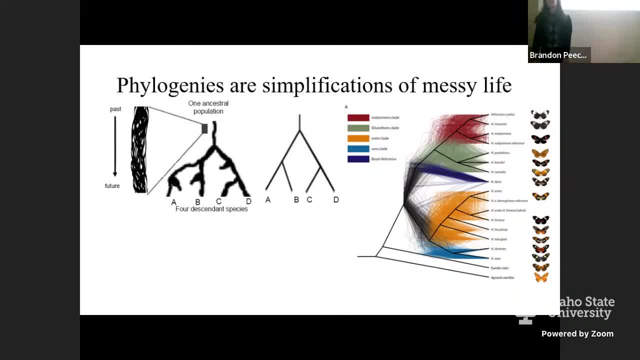 confident in of the relationships amongst all of these different- you know different- species of different heliconius butterfly. So one genus of butterfly. there's a bunch of species in it. Here's how we think those species are related. The black lines show you the phylogeny You can see. 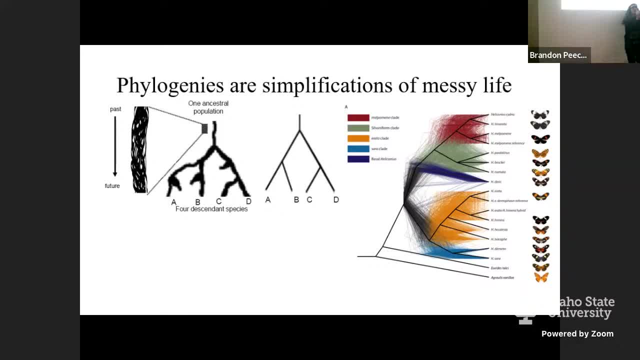 some places it's unresolved, like up there in the green, there's three branches coming out of one spot. That's not so great. It means we don't know something. All those rainbow colors are different clades. We're going to talk about what clades are today of these butterflies that everyone's 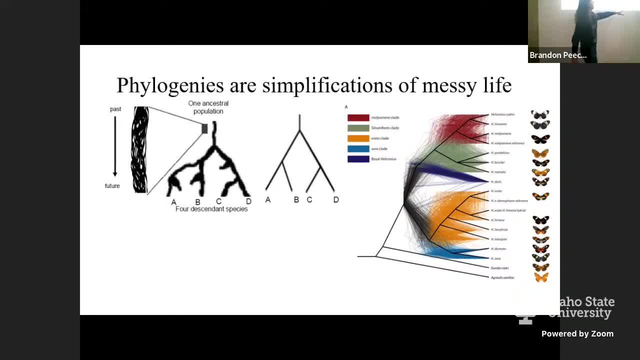 confident are real biological things. But what I love so much about this figure is that it shows you the absolute power we humans have at discerning relationships. now, All of those like crazy squiggle lines are the exact same set of butterflies looking at this gene. the exact same set of 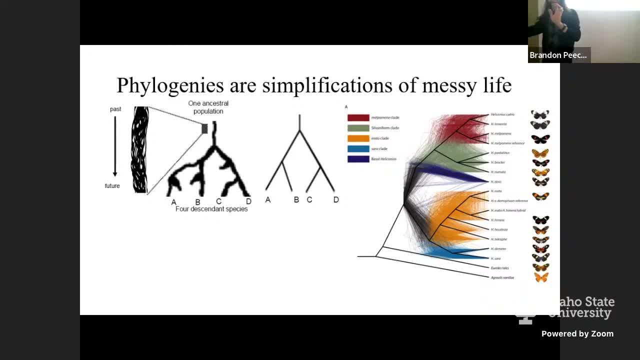 butterflies, looking at this gene, that gene, a different piece of the genetic sequence of all those butterflies. And so you can imagine, right, if it's a gene that codes for like pigmentation, the gene that codes for like how their gut forms, and if the gene that codes for the proteins in 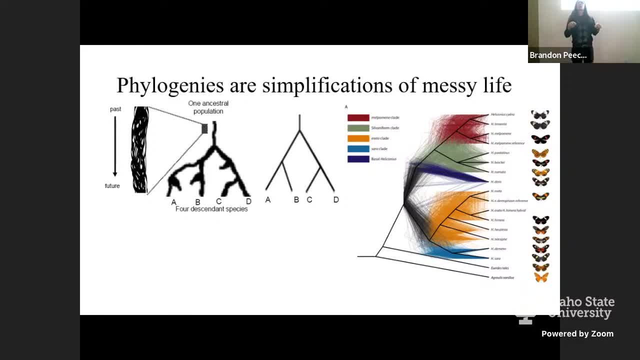 their eye lenses. all of those genes, you would expect would use the phylogeny of these butterflies, usually have the same arrangement with each other in terms of how they descended, comparing the same gene across all the different species. And so, because modern biology is so, 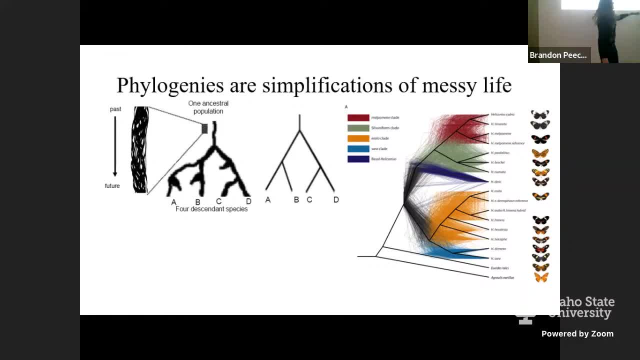 crazy. we can like full genome sequence, all of these butterflies, and we can see that like there's like a cloud of probability almost if you get so much data. And I just think it's really cool for you guys to see that in some, in almost all cases, what we might call the real tree. 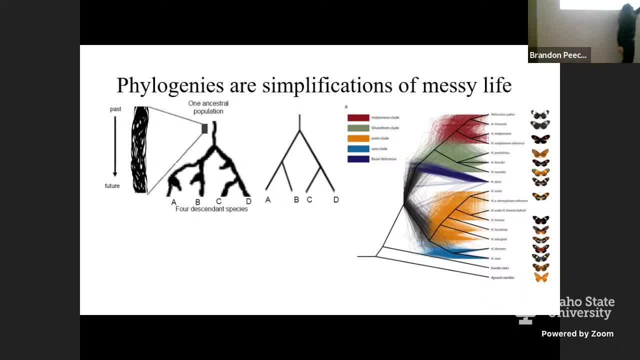 this thing, which we hope is the real thing, matches up with almost all the kinds of evidence we can gather, but it's not perfect. So if you guys just do me a quick favor and talk to each other and, like, make some observations about this butterfly tree, where you see things that 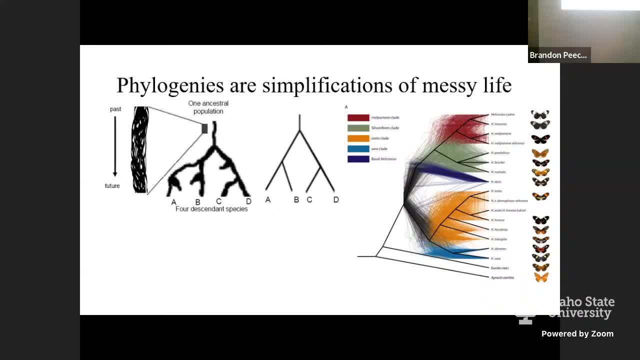 look like they're not perfect. it doesn't matter, you don't know about this butterfly or about the genes, you just use your color vision. All right, can I get some observations here? Not looking for any one thing. Yeah, actually the purple doesn't really have any like. 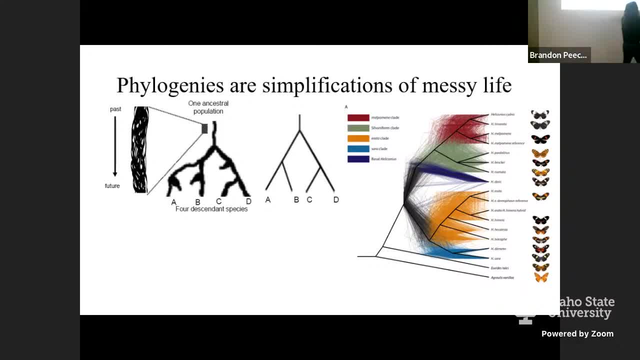 lines that are strong, I don't know Whatever. this is the thing. So what I think is cool here is you can see that like there's a pretty strong purple like this, So most of the genes in this butterfly, which, as a species, is all by itself. 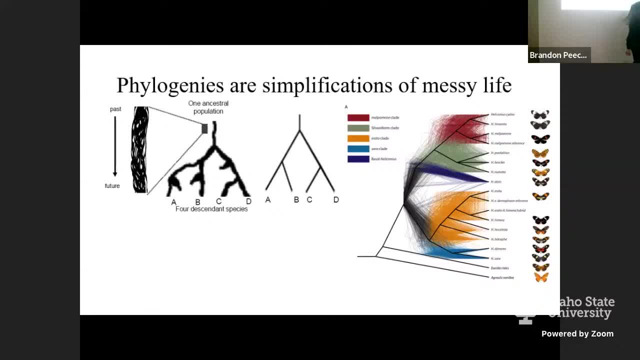 probably on that side of the bigger split within the genus. But what's cool about this is like: yeah, there are a few different genes that if you sequence those genes, it pops out over here with this, with the orange and blue group instead of the green-red. 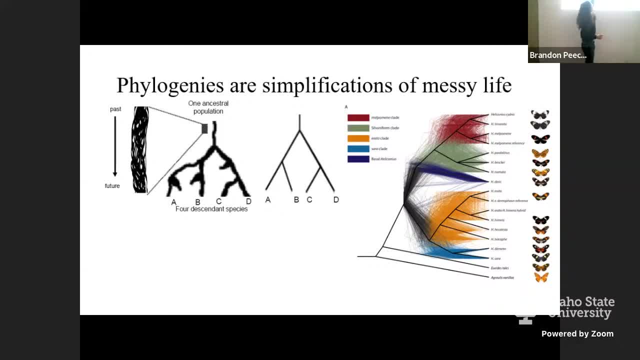 And that's just interesting. If you imagine life as messy, where populations are kind of going back and forth with each other, this butterfly is, we would say, early diverging relative to these other ones. The other, the red and the blue one, sorry, red and the green up there, diverge later, And so 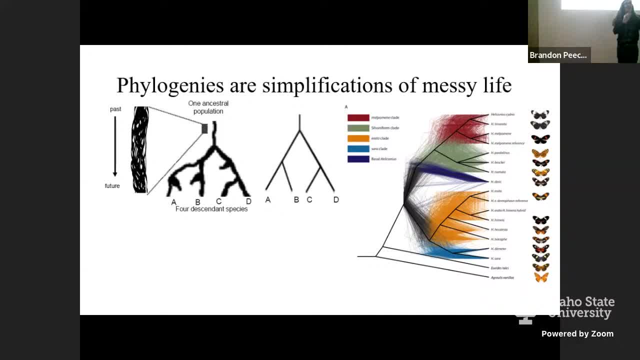 this purple one probably goes up with that. We can be really confident about that. but there's actual little teeny bits of evidence and it makes sense if you think about how populations really breed and move through each other, where some of the different genes you might sequence might. 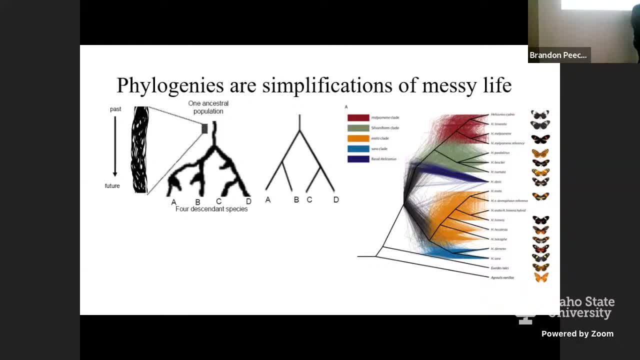 give you a slightly different result, It doesn't mean that that answer is like wrong. I just think it's important for you guys to see that, like when phylogenies are made today with genetic information, people are like running millions of data points and then they're running like 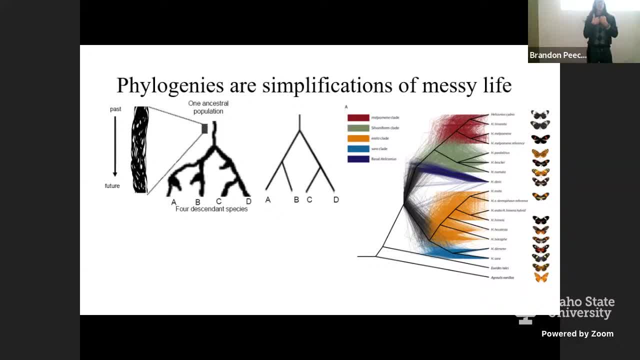 probability estimates. When I do phylogenies and when you guys see phylogenies in this class that are based on anatomy, it's all like four gills, six gills, Yes or no, Like that's the data We have and that's what most biologists have for almost everything we've been talking about. 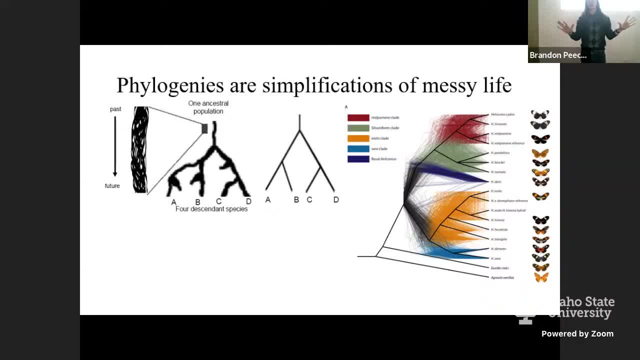 I just want to make you like go like this, oh gosh, when you see like how powerful genetics is. And so what's great is like when four gills, six gills, makes a tree between sharks and trout, and I like that tree. What's amazing is that when a geneticist comes through and like carpet bombs, 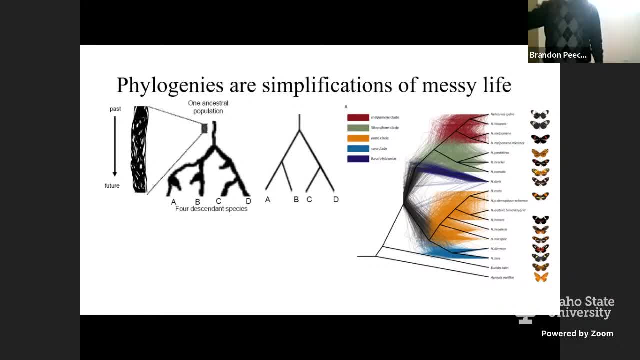 like six million more pieces of data, and they all say the same thing. we can be like: that gill thing worked out great, And so there's other times when the gill thing is going to work out badly and I'm going to tell you about those. But so anatomy has great explanative power. but 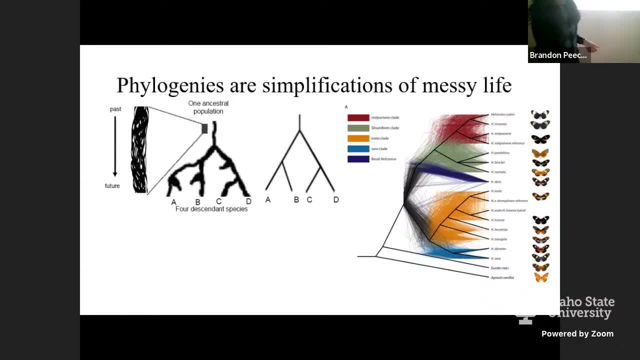 when lines of evidence interact with each other. that's when modern biology really is kicking butt, And so this is just another figure that I remember being an undergrad and being like, really like calmed by because it was so interesting. So this is the paleontological figure, that's. 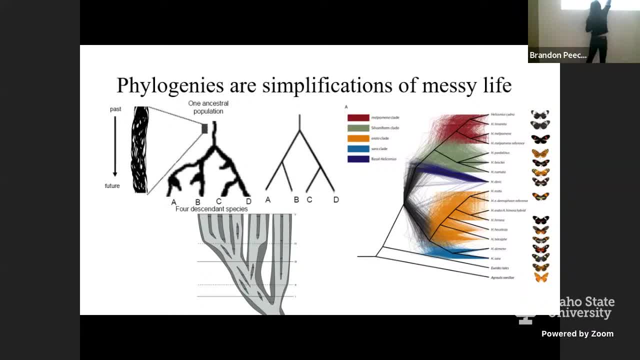 supposed to be showing you. here's an ancestral population and here's a bunch of species alive today, and these are all different slices of time. You can imagine like today, 10 million years ago, you know 15,, 20, and it's supposed to be like: look at how the populations of the 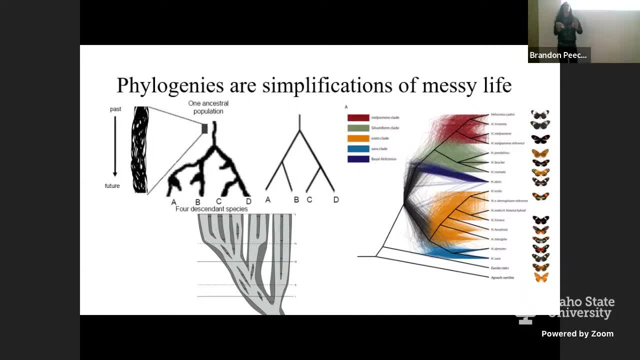 light, gray and for moments of time there's a split, like there's like an island, almost like in a river, and they come back together. And so when you guys read into a bio and you're learning about speciation, like this is the actual split between this big lineage and this big lineage that maybe 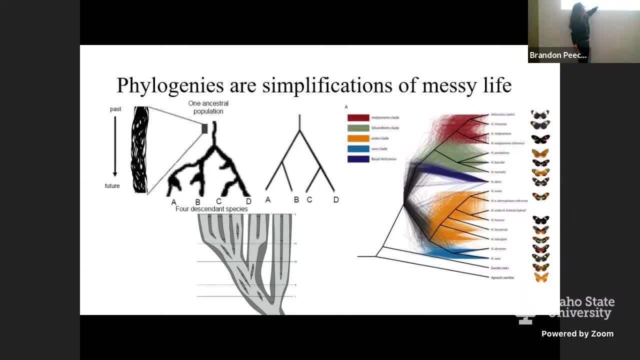 these are both two species. Within each species there's populations, but even if you go back far enough, there's moments when like this didn't become four species or something like that. This is all just kind of woo-woo-y. I just really like it and it's my only chance to really give it to. 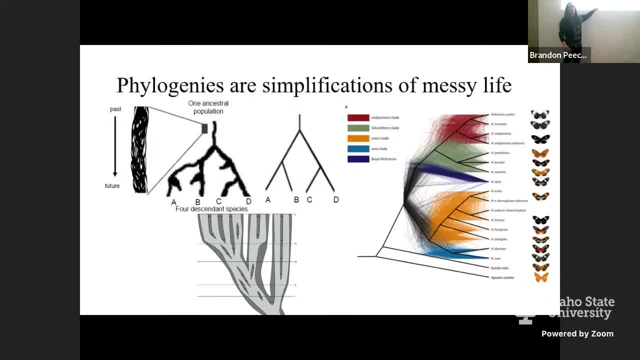 you guys, Right now, on the surface of this planet, there's a bunch of species that are like: oh. there's a bunch of species that are like: oh, there's a bunch of species that are like: oh, right now, on the surface of this planet, this is happening Like I guarantee you if you were. 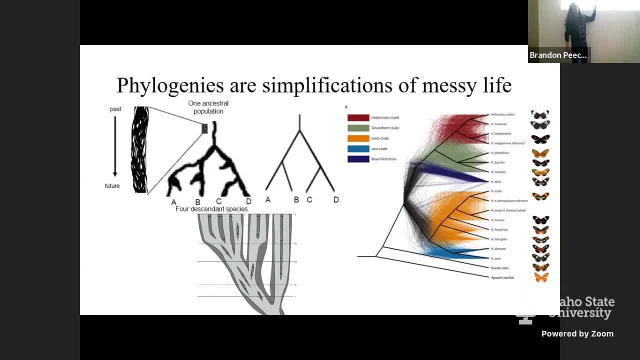 like cut crows or bears into their constituent, like grizzly bears into their constituent parts. it's going to look something like this: There's gene flow between some populations, absolutely not gene flow between others, And we all call them- maybe you know- ravens. but come back in. 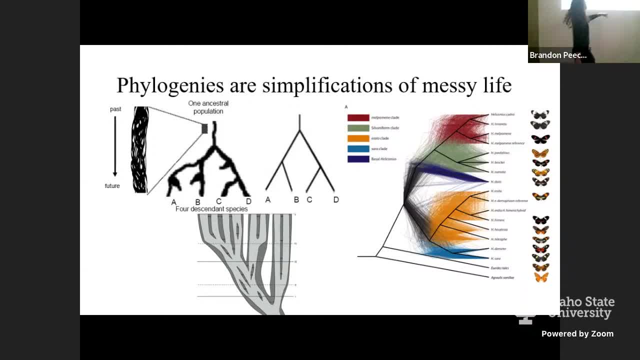 five million years, there might be a couple. I just think that's really cool and really important. Whenever we talk about it, all I want to give you guys is these dumb straight lines. I just want you to have them. I just want you to have them. I just want you to have them. I just want you to have. 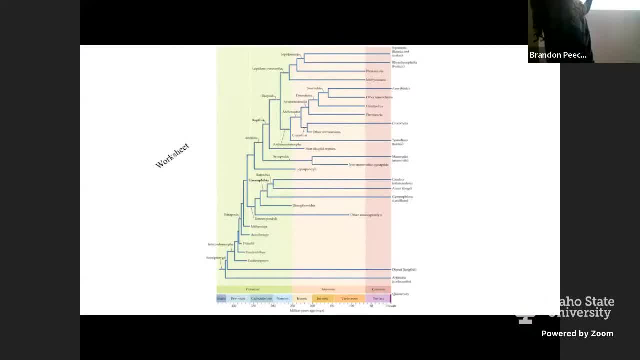 it in your hearts what it really is. That was how I wanted to end on Thursday, but we ran out of time. That's why we're kind of starting with like a thing like that: Okay, from now on for the. 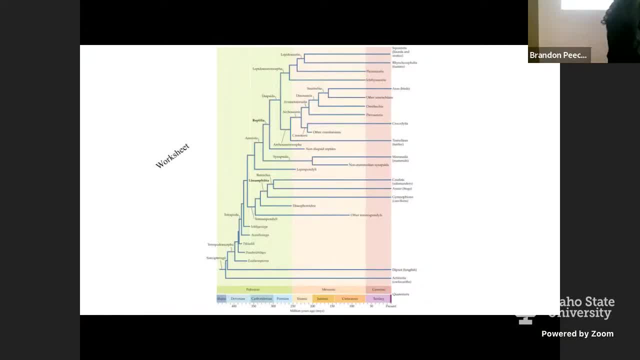 well, for the next 25 minutes, half an hour, maybe you guys are going to be working on. that was terrible, wasn't it? Well, I don't want to do it all the way. I'm going to give you guys a worksheet to do with each other, So you're going to read it. 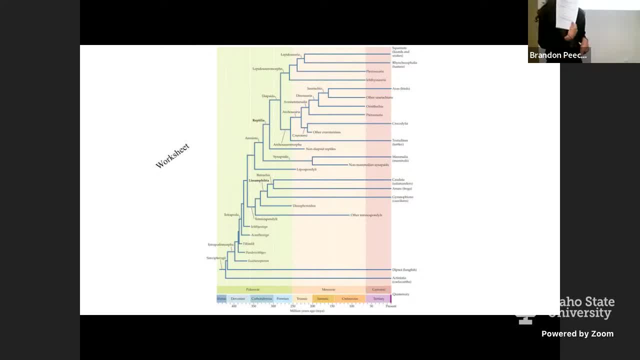 It says right at the top: if you don't know what any of these words are, that's okay. You're not coming to this class, like I'm expecting. you already know all this stuff. We're going to learn it, but I do suspect that some of you do know some of it, So that's where. 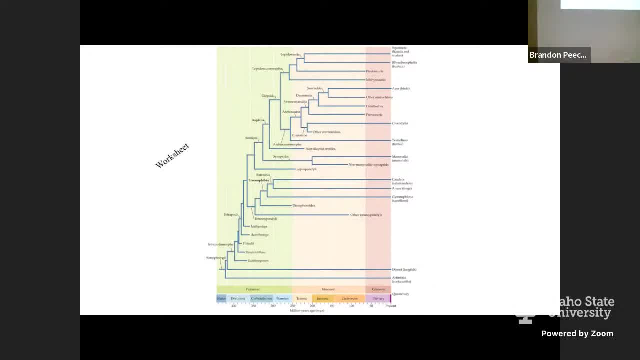 we're going to start. We're going to work in groups of like three or four. if you can, Don't work by yourself and work with at least one of the person, All right, let me know if there's any spares needed. 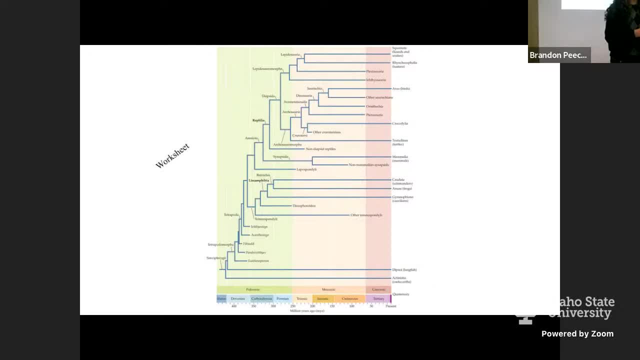 Yeah, groups of three, groups of four, Great, great, great. Okay, everybody have a sheet, Okay. so on one side of the sheet there's some like introductory kind of stuff. This is almost like a survey. You might not know what anus is, and that's okay. 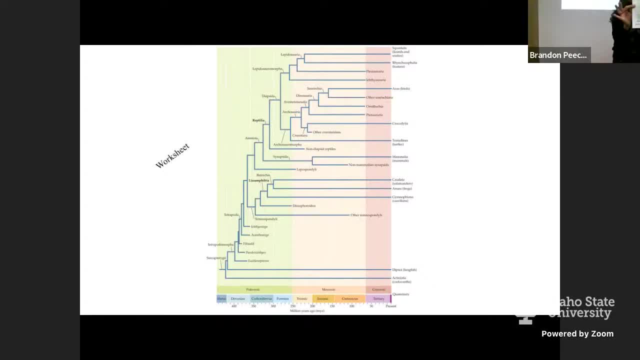 I'm giving you this on the back. This is a figure from the herpetology textbook. If you ever take Dr Peterson's herpetology class, this is a figure from that book. I use this figure because I just love it so much. It's definitely TMI for you guys. You don't need to. 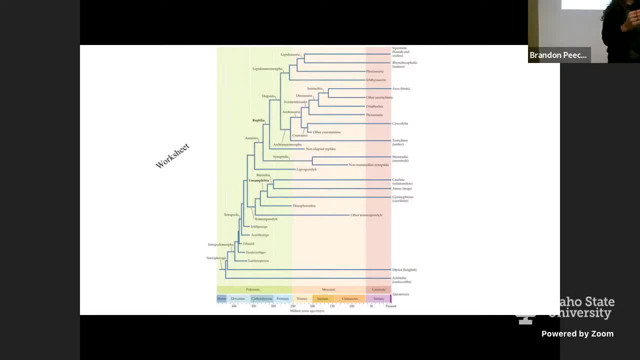 know all this stuff. It's way too much. What I like about it is that it's a phylogeny that is mostly. well, it's all vertebrates, It's the lobe finned fishes, so something like the coelacanth. 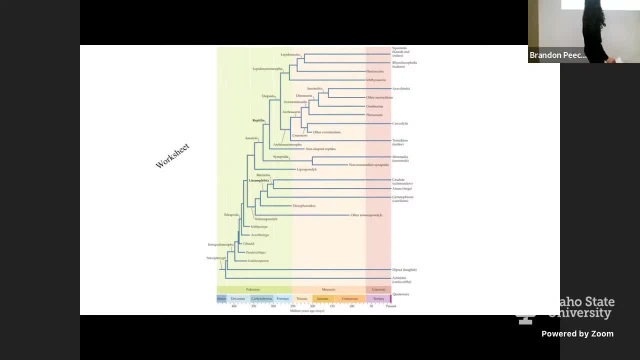 plus us. What you are seeing here is a phylogeny, and then this is some paleo, but I'm sorry, I can't help but sneak it in. So geological time is on the bottom of this chart. So there you are. 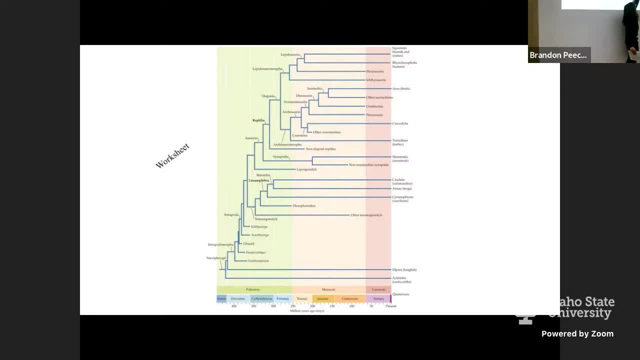 there I am. We're sitting here in the present and things like coelacanths and salamanders and turtles are living organisms, And then the phylogeny goes back through time, and what I like about this is that you guys will get to keep this, and it'll be a little way for me to sneak in the 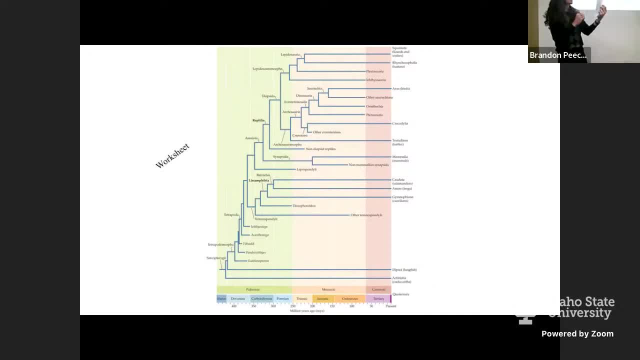 fact that you'll have some idea of the geologic age of some of the big groups of vertebrates that we're talking about. All that matters to the worksheet is how the lines connect. All the things that are back here are like extinct things. You can ignore those. I don't care. 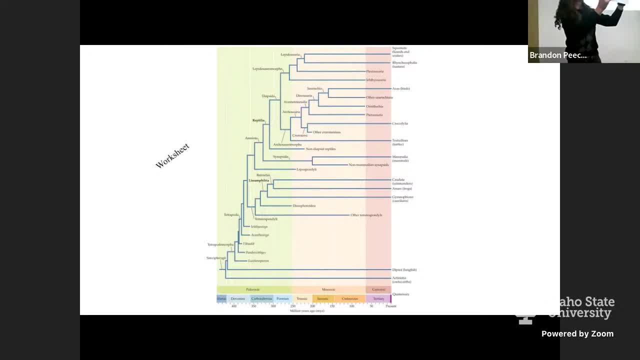 Focus on the stuff that's alive and use this as just your thing. you can squirble on for answering the questions on the other side. And again, please work with each other. I'll be walking around Here we go. 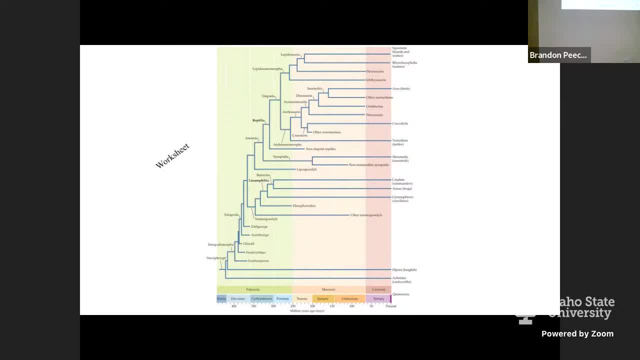 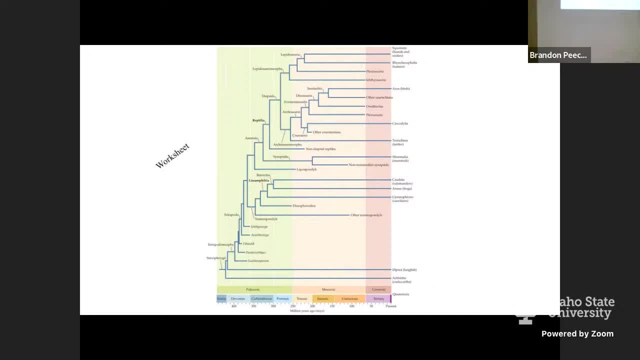 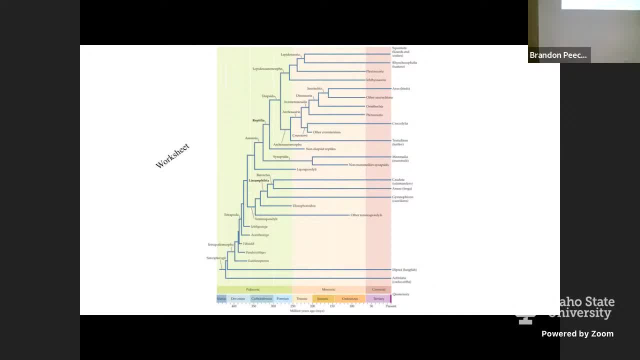 Thank you. Are we? are we feeling like we've made some kind of progress? I'm sensing the slowdown. What if I said I mean no, I definitely don't. Okay, So over here I've recreated this figure. 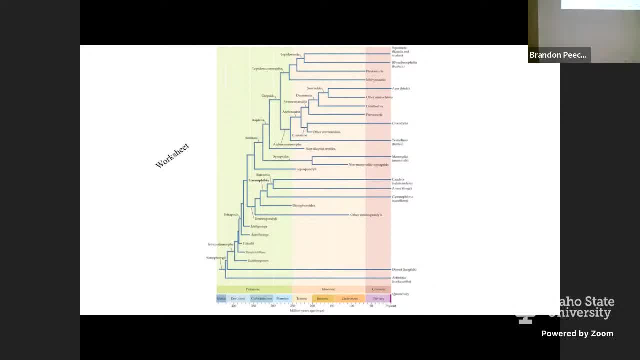 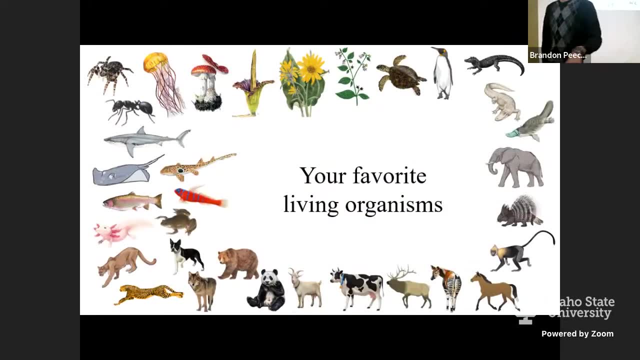 but I've taken all the paleontology out of it, So it's just what's alive right now. So it's the same thing, same order, over there And then over here. I just picked a few. I thought I'd do them all, but it's too many. 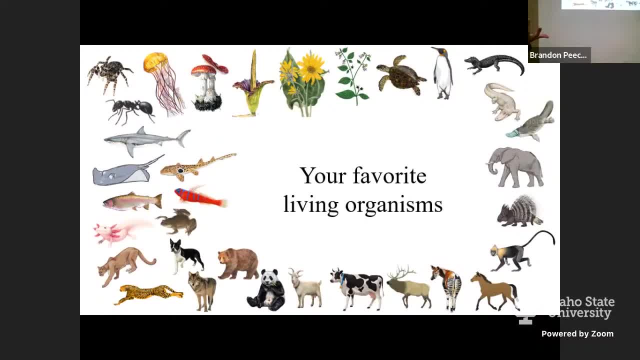 I've just your guys' favorite stuff, So there's a phylogeny. You can make a phylogeny of anything, So it's not weird to have jellyfish and flowers on there with all those dogs. But anyway, there's a phylogeny of your guys' favorite stuff. 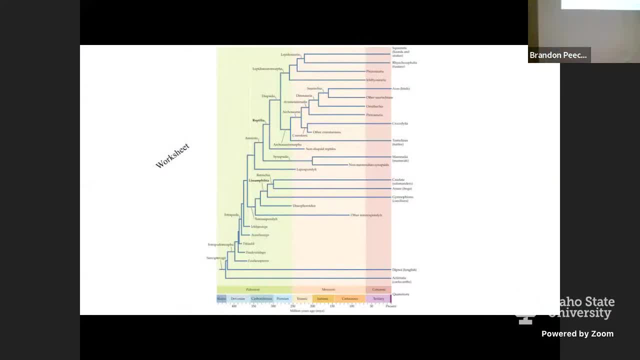 There's a phylogeny. that's a simplified version of what's on the worksheet. Can you two groups go up there? Can you two groups go up there And all seven of you, or whatever it is now just do number one and number two. 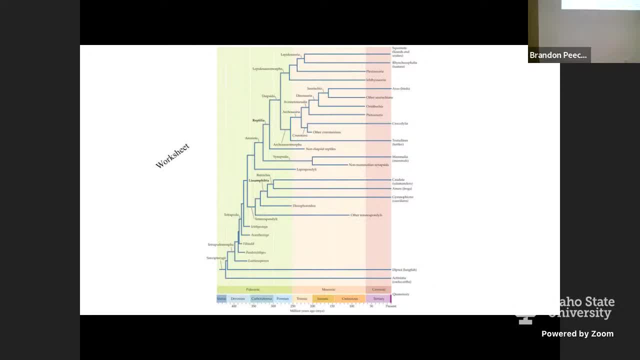 like marking on this tree, So those things. And talk to the other group. Talk to the other group. Let's see what we got here. It's definitely okay. This isn't bad. I don't think we can hold it. 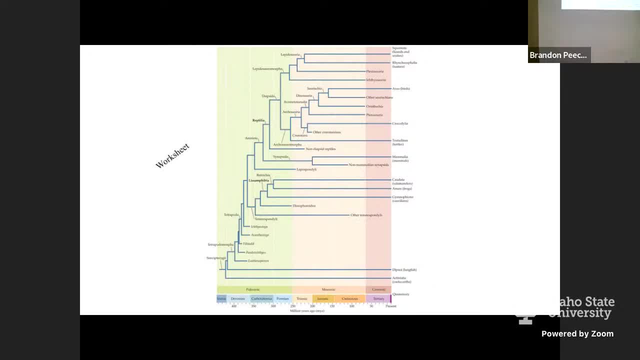 I don't think we can hold it. Okay, Oh, what Are you kidding me, Luke? Yeah, Yeah, So you want to? you want to do it? All right, Make sure everybody's included. Everybody agrees. just to say: 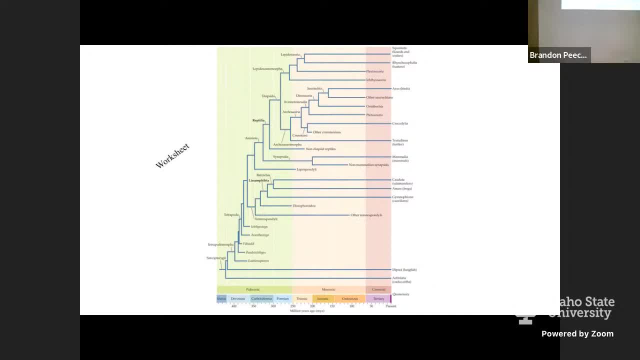 Okay, Sorry, Go ahead. I don't need any superstars circling everything. I'm so excited I already have an idea of what's playing in the show. Yeah, I'm sorry. Yeah, Well, everything Like, if you. 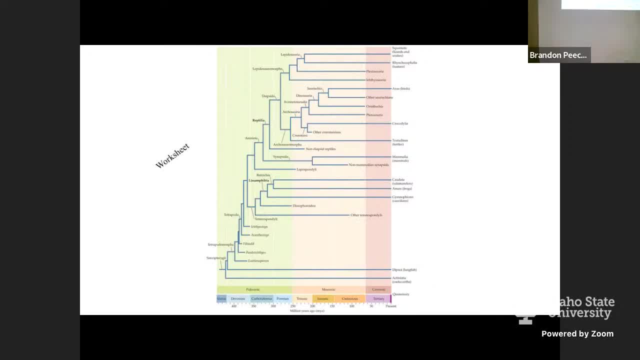 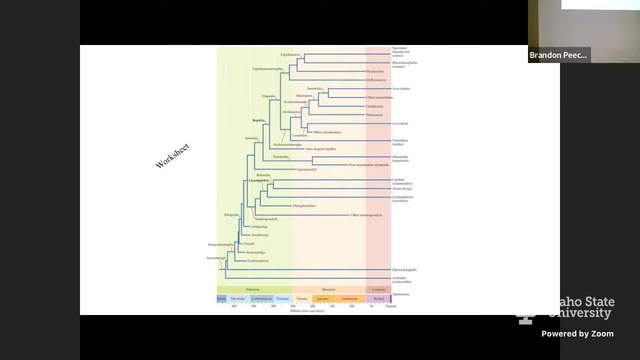 Yeah, it doesn't matter. Is it good in here? It's not bad, I think. All right, Yeah, Yeah. So you like one of these things, Yeah, Yeah, yeah. Would you be careful that it could, like, have some but not all? 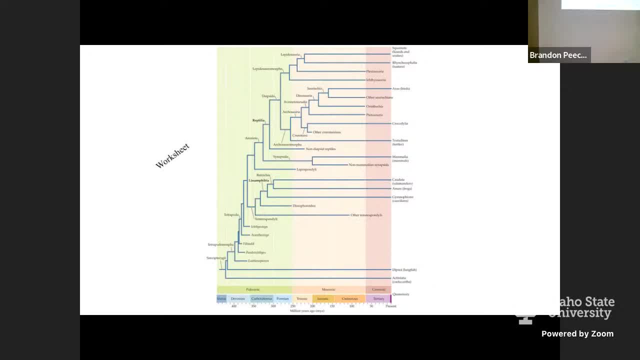 So like if it doesn't, I mean like the headphones and any other things, Perfect walls, Like sister groups. Okay, let's see They could be wrong. I don't know. That's easy. That's the perfect sister group on that tree. 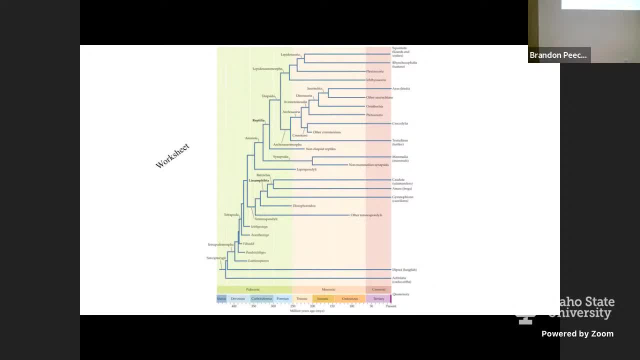 Yeah, What a great, what a great badger argument. It'd be like: where in the world would I be able to see a monkey in a park at the same time? No, but I mean like where Continent scale And zoos don't count. 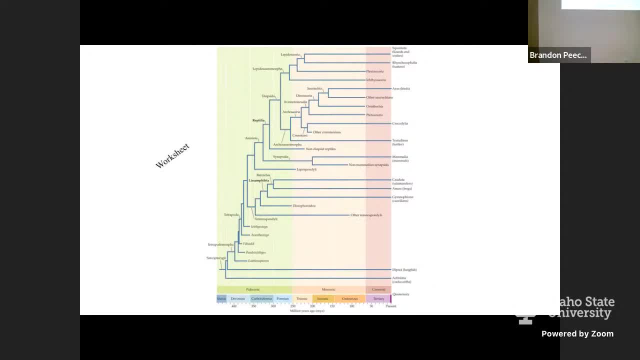 I'm not saying anything, I'm just like thinking like: hmm, I mean, it sounds like a monkey mind, It sounds like a monkey mind. I mean, it sounds like a monkey mind, It sounds like a monkey mind. It sounds like a monkey mind. 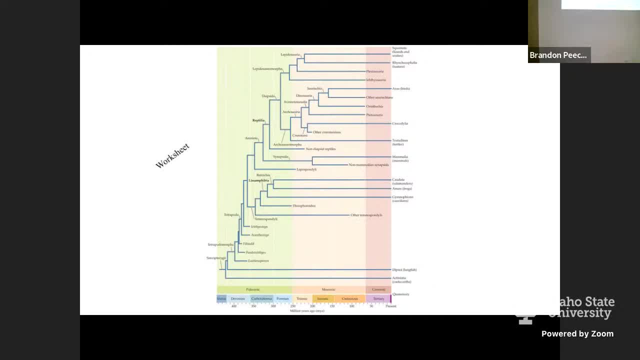 It doesn't say what kind of monkey. Yeah, Monkey's parapsychotic, which is really people. That's interesting, See, this is. this is why it's like one point for the answer and five points for explaining your reasoning. 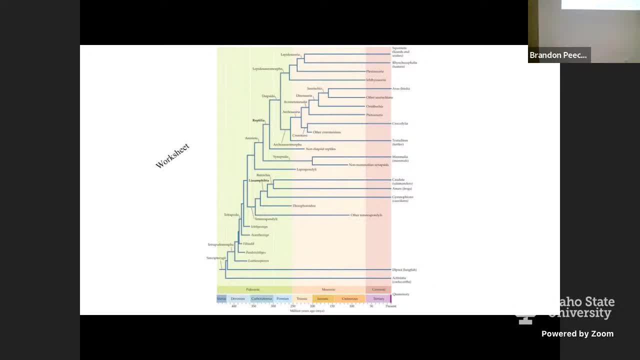 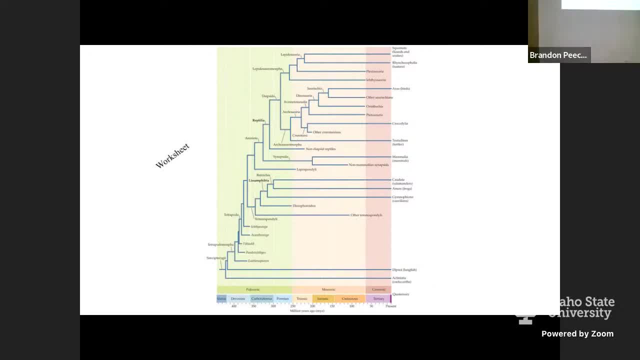 Yeah, That's, that's um, Uh huh. I was like, oh yeah. I was like oh. I was like, oh, It looks like Oh, Yeah, Okay, Yeah, Yeah, All right, I think it's the same. yeah, four or five, but yes. 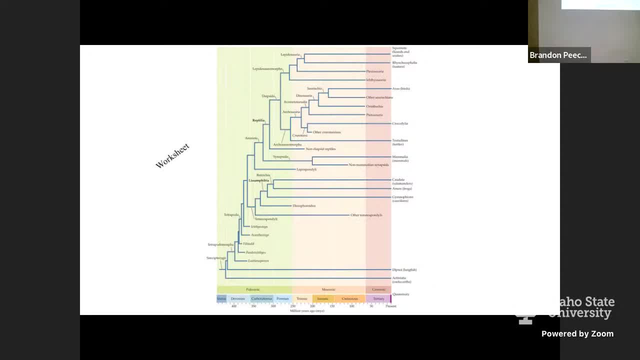 Yeah, they're literally everywhere. All right, I'm feeling like we've got number one and two at least. what's important? Yeah, Okay, great, Do me a favor and swap with each other. look at the other people's tree, make sure you're like that. 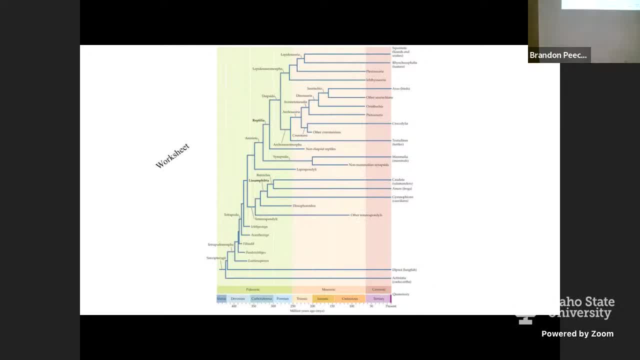 It's copacetic, I get it. Or if you don't, that's okay too. Where's the alligator? I'm sorry, Alligator, What are you putting? Alligator, I'm not even, I'm just doing bow and point. 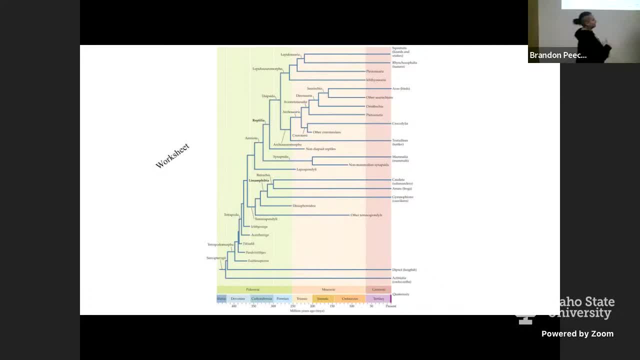 Yeah, it is. I'll call back to one of my famous cop-outs: B-A-U-P-L-A-N. I don't know how you spell bow point. Do you agree with the labels that they put on there? Oh, okay. 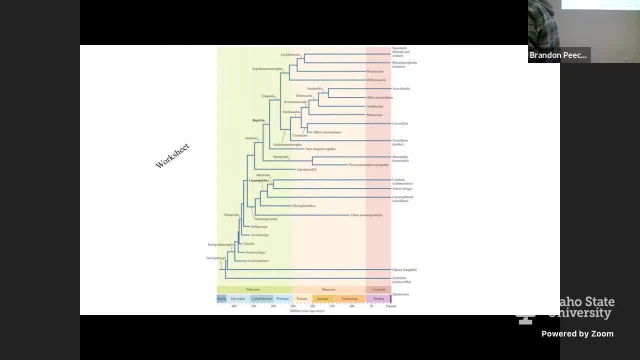 So This one will be a different model of a Pakistani. Oh, okay, So this one. Hello, we have right here in the audience. We actually brought her to school, so we'll go ahead and share it with her. Oh, all right. 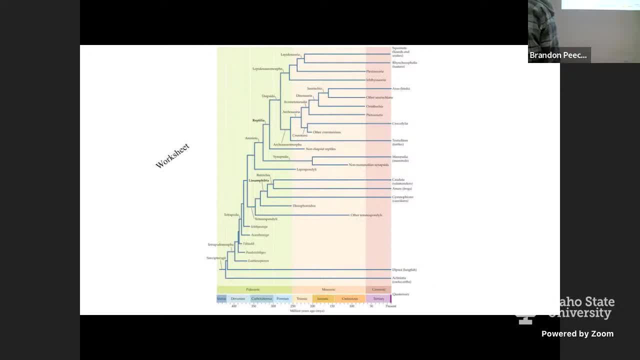 It is their class. I think I put each of these words on the paper on that in your lab. Oh oh, good job. Thanks, We'll see how the reviewer's thinking We're discussing turtle pylonging. It will not be a disputed fact. 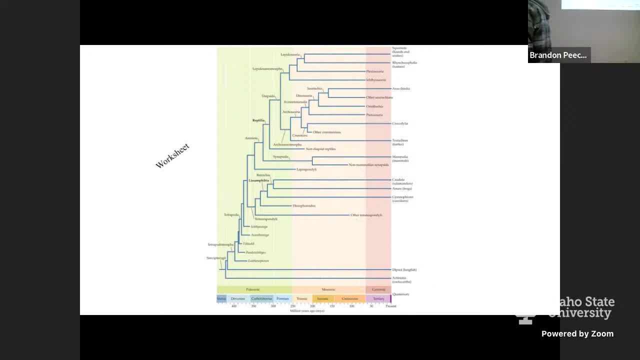 Relax, It's getting there. We're on one of them, We're on Scott's side, All right, It feels like you guys got it. I have only been looking and I think we're not understanding or have questions about each other's trees. 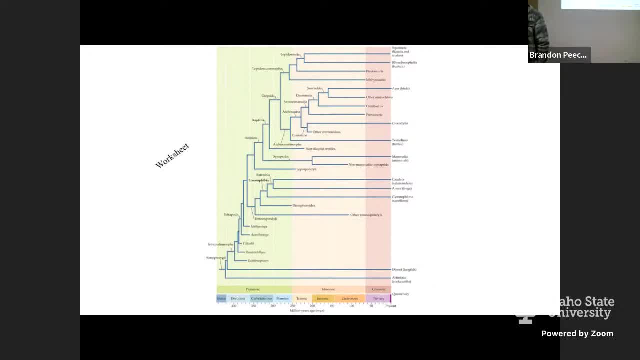 That's great. I haven't actually looked that hard so I'll make sure nothing looks problematic. Monopoly through four: That's right, We have a second here. I started Awesome, awesome, awesome, awesome. That is awesome. 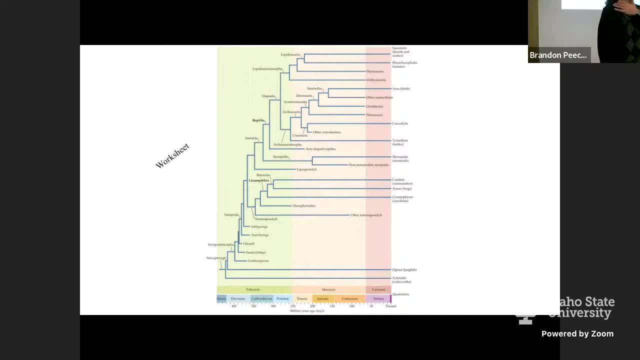 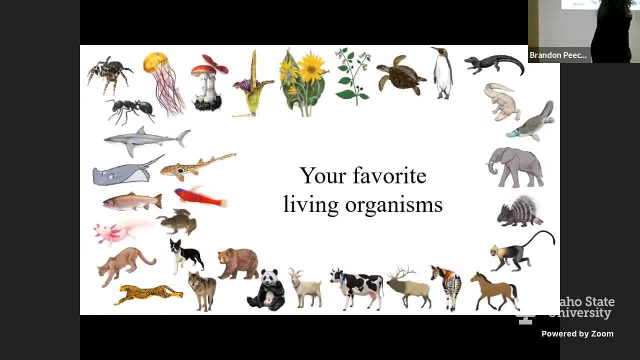 The hive mind, I think, has mostly gotten stuff up there in a way that makes sense, but now we will give you some backing as we go forward into this stuff. Anyway, you've already seen this. That's your favorite. I just wanted to show you this because you haven't seen it yet. 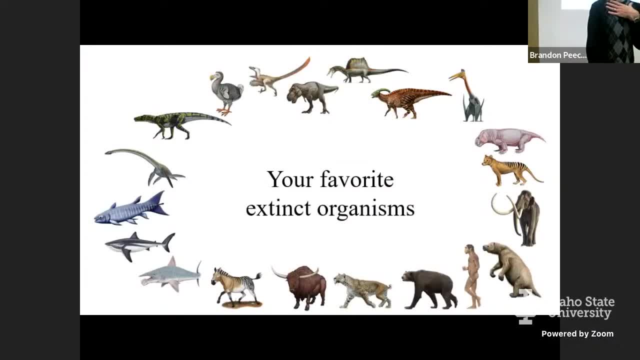 Here's all the stuff you said was your favorite extinct stuff. It always makes me happy. No point for class, I'm just showing it to you. Congratulations on whoever said the haven horse. you're for sure from Idaho, I don't know who it was. 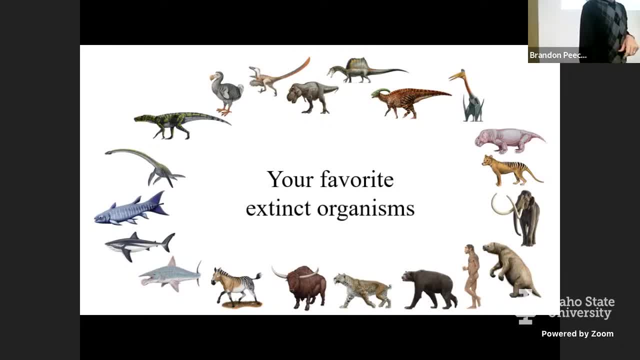 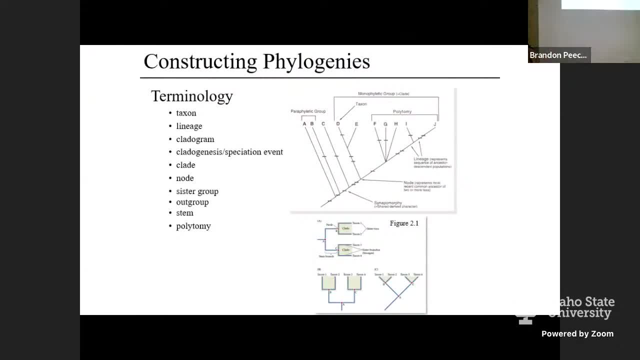 You're an Idaho person for sure. Cool, Good stuff up there. Anyway, There are going to be some slides. All these slides are, of course, going to be on Moodle. You guys can go back and check on them. What I like about a lot of these diagrams is they go out of. 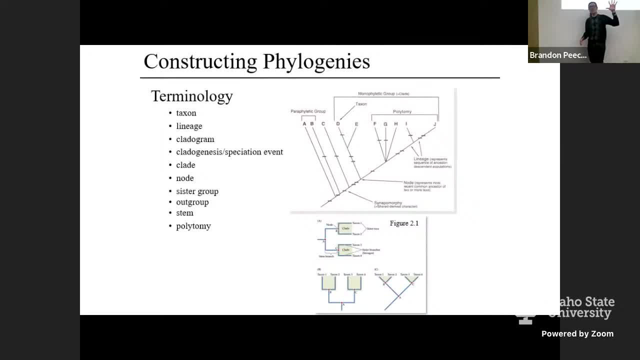 their way. to make everything really explicit, The information on them is contained Three weeks from now, when we're talking about the evolution of vision and I say something about a polytomy or whatever you're going to be able to. I don't remember that one exactly. 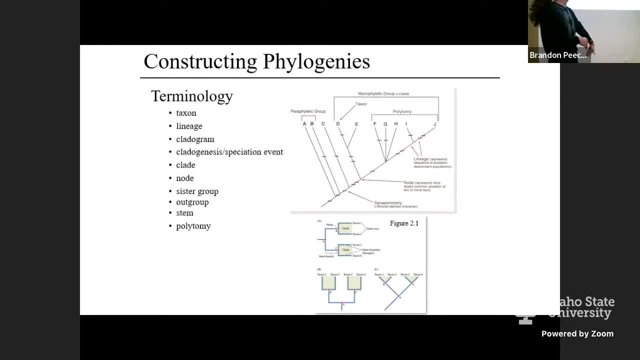 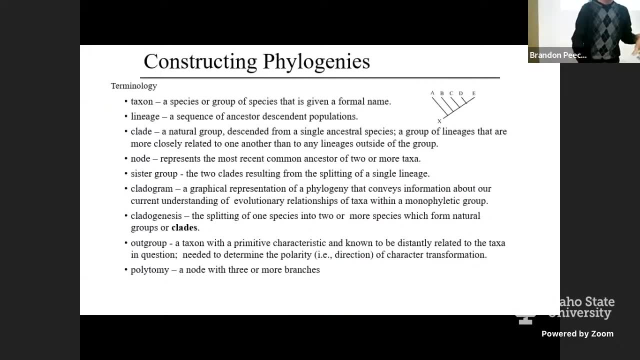 These slides, I hope will be able to be helpful to you. There's a whole bunch of terminology that comes with this stuff. We're not going to use all of this. on the slides All of these terms are defined. You can always come back and look at this. 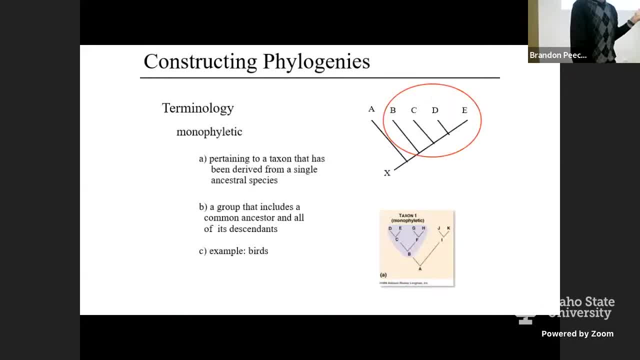 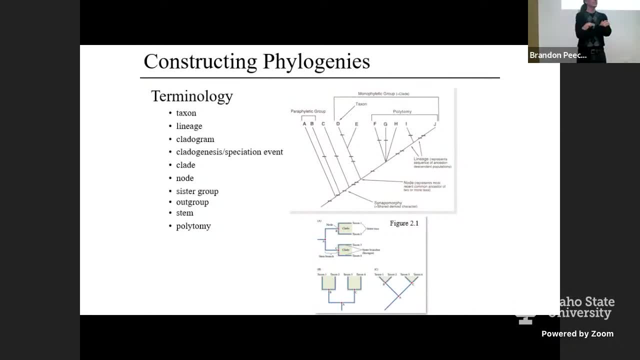 I'm not going to spend our time here in class reading this out loud to you, But I want to go over the couple that were on the worksheet, at least because I think they're important. Can I ask you to volunteer on what is a taxon? 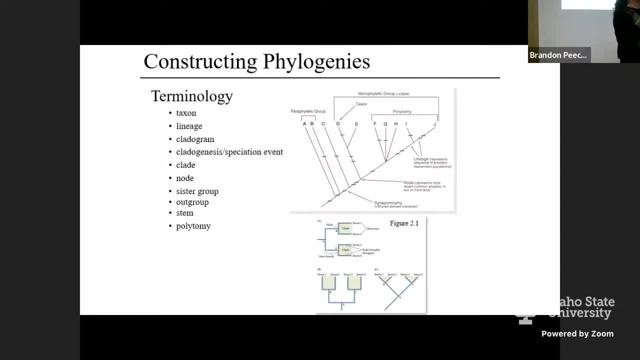 That's number one. first thing, It's a group, it's not you by yourself. What does your group say is a taxon? Do we need to teach each other? Yes, Amy, What's the taxon on this tree here? 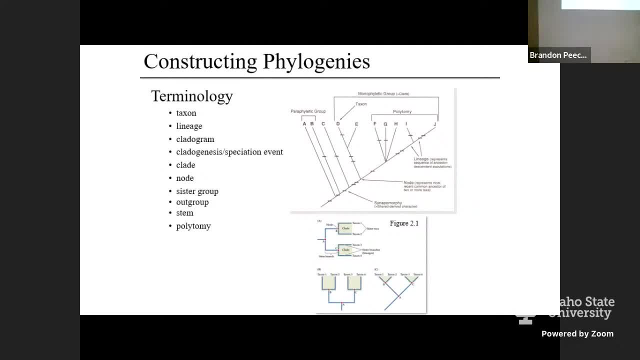 We said jellyfish on there, Jellyfish, Any of them. Any of these things is a taxon. Any of these things at the top of a phylogeny, a clay that has a name, is a taxon. Any label is a taxon. 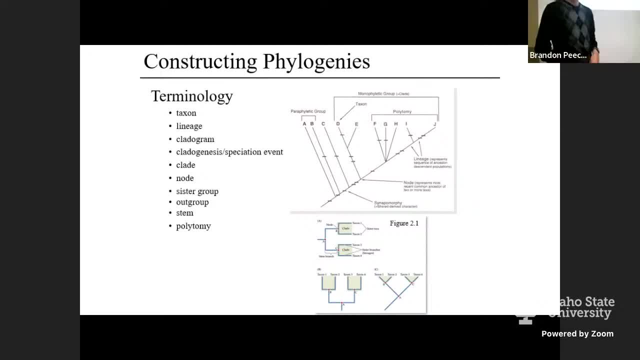 Taxon is just a group of organisms, Taxa is plural. That's that Lineage. it looks like both groups did something similar for lineage where you drew a line going back, which I think is great. There's a lineage there. 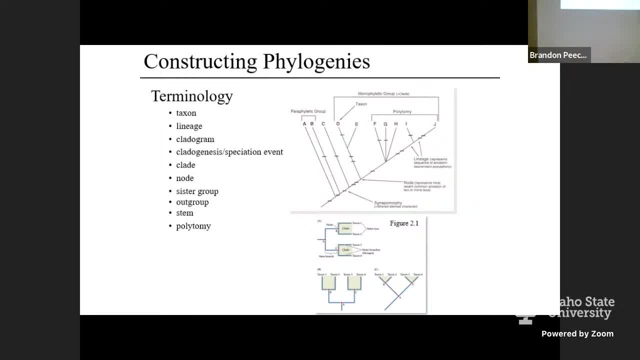 Can someone tell me a little bit in detail about, for instance, this group? what is this lineage versus this group, This one versus this one? I just want to make sure we're all on the same page. Tell me about this lineage. 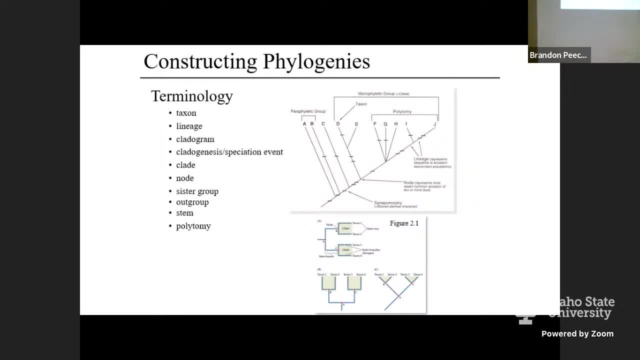 I don't know if you're hearing me specifically. The way that I was thinking about it was: it's not a bunch of different ages. just if you take mammals, for example, and just follow it back, This gigantic tree, you're going to learn this. 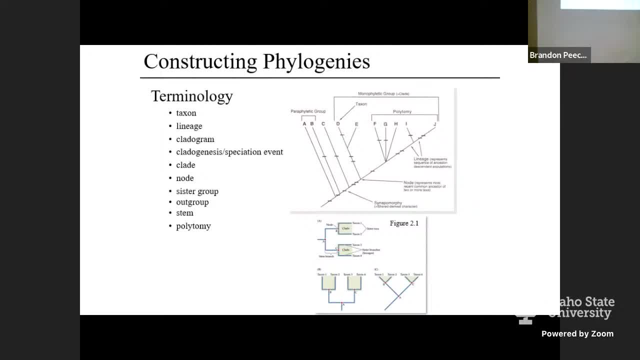 so I'm going to say it for the first time: On this tree of Sarcoptorygian, this mammal and this right here, this horizontal line is the mammal lineage. Then what is this one? The lineage that contains the ancestor of mammals. 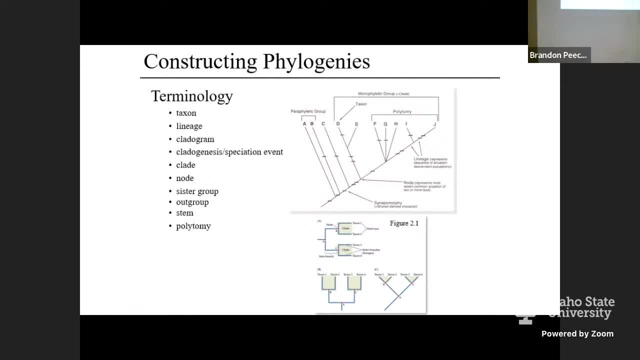 but also the lineage that contains the ancestor of all these guys, which have their own special names that you guys definitely already know Because they're reptiles. But the point I want you to make is- it's this hard thing to think about- This is the tetrapod lineage. 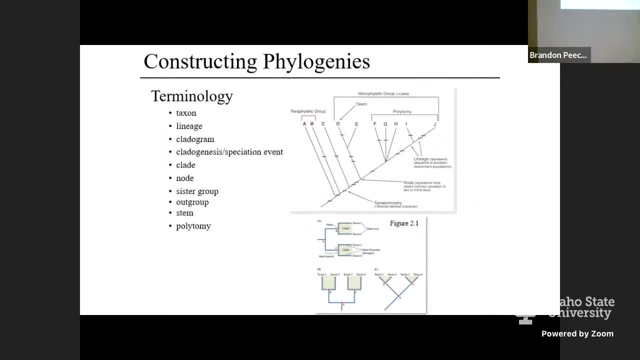 This right here is called tetrapoda, and everything after this has four legs. This is the tetrapod lineage, but the mammal lineage is contained within that little back part. Does that make sense? There's one population here. there's one population here. 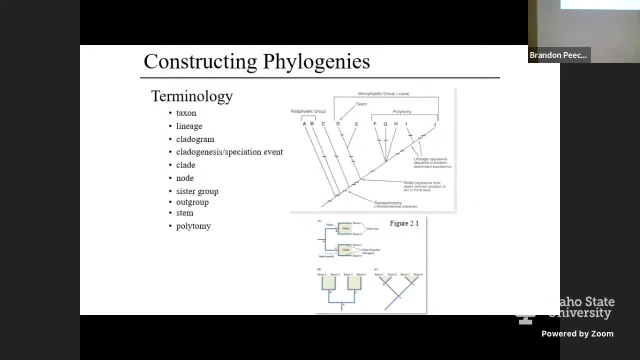 there's one population here. Mammals have an ancestor that runs through all of them, but as you go back farther and farther, it's joining up with many other different things. This thing is not furry. The fur has an equator. 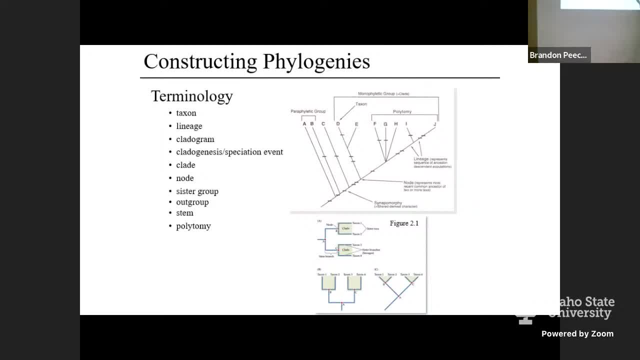 That's like lineage, so it's like the line on the tree. I'm going to be drawing phylogenies that are a little bit loopy- Mine are always curvy- because all that really matters is the branching between the different lineages. 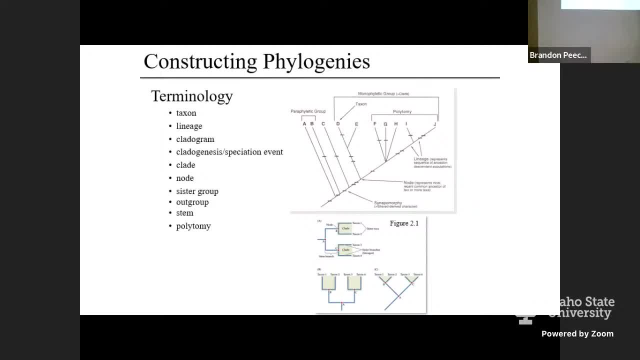 That's all that matters. You guys might see this a lot, these diagonal lines making the phylogeny. It's the same information When the trout and the cow and the coelacanth last week was all diagonal, These type of phylogenies where there's right angles. this isn't different. 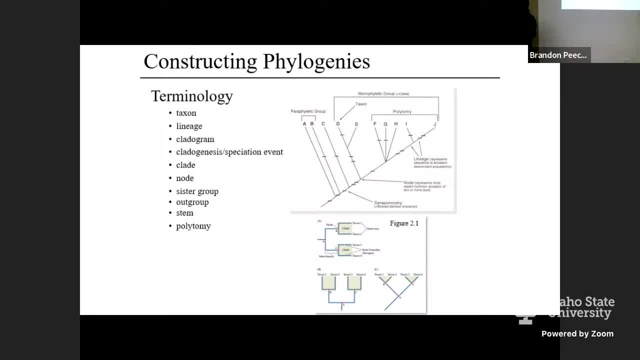 What is amazing is that people who do biology education have done pretty rigorous research. High school students and undergraduate college students learn phylogenies easier when you have it be boxy, which I just think is amazing. I'll do this sometimes, but I'll also do that sometimes. 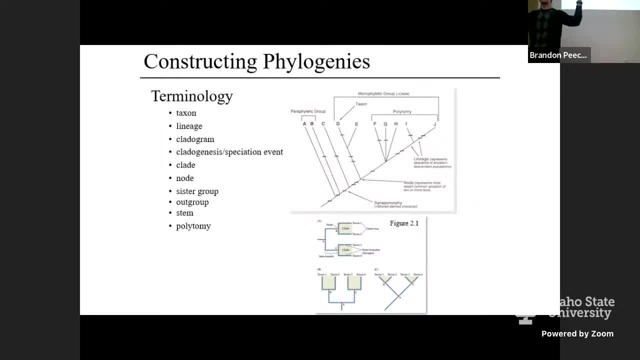 and you guys will see soon enough. most of my phylogenies look like this, because I'm trying to fit it all on a slide, But all that matters, of course, is the branching. You can diagram it in a bunch of different ways. 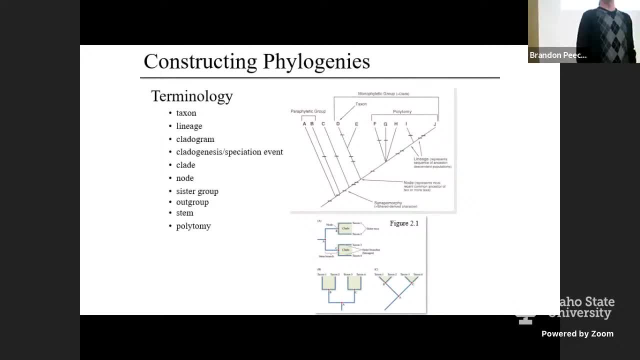 Those are the lineages. What's a clade? What's an example on your tree? The Tuatara, The Tuatara. They have a common ancestor. right here There's a whole bunch of words we can talk about now. 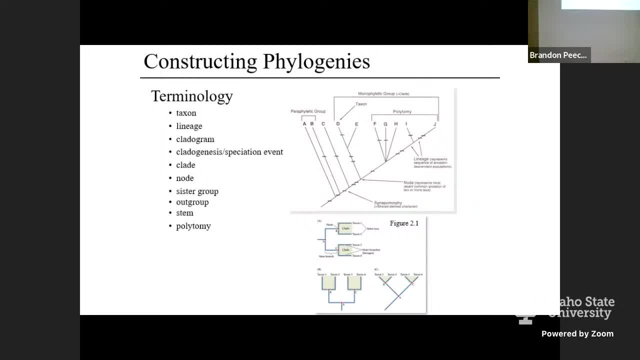 What do we call this thing on the tree? That's a node. The node that's the common ancestor between these things, this and this one. what would we call these things together? The other sister, any sister groups, share a node. That node represents the common ancestor. 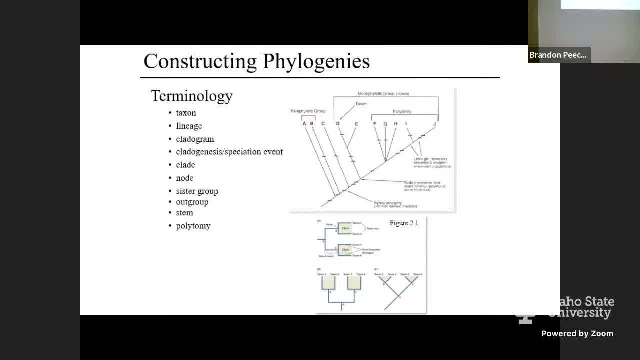 The common ancestor and all the descendants makes a clade. Wow, You see how these things all mean really similar things. I'm just trying to make sure we get it all straight. Those are all labeled there on the board. Great, There's a node. 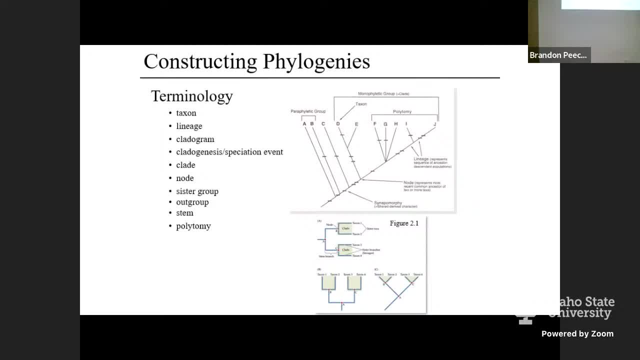 Frogs and cow-managers are sisters- absolutely. Birds and crocodiles are sisters- absolutely. That's crazy. Looking at this, or looking at your worksheet, or looking at that tree of your favorite stuff that I just threw up there. 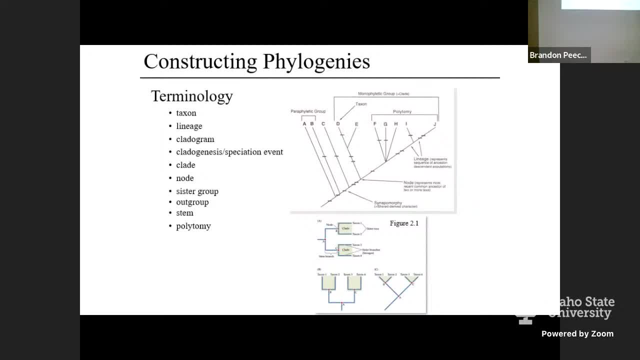 totally for fun now, Any relationships or things that you're like? I don't know about that or I want to know more about that. Alligators and penguins. Alligators representing crocodiles, penguin being the only bird anybody wrote on their favorite animals. 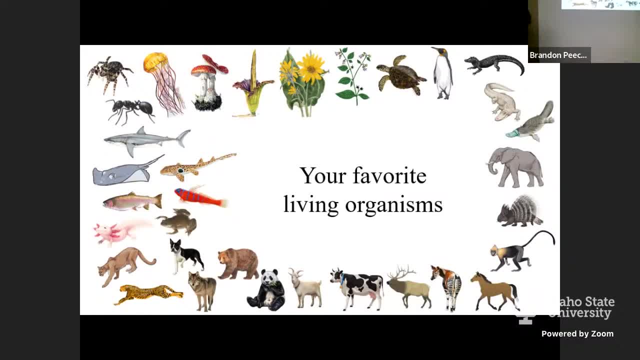 This is. birds and frogs are each other's closest relative. This node right here has a name. You guys will learn it. The only other reptiles people said, besides another gator, was a turtle. Here's your node that represents all reptiles. 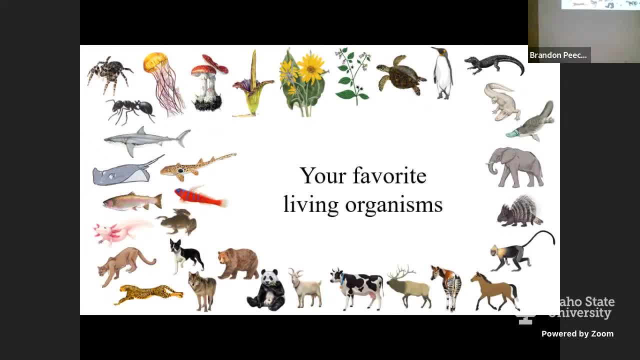 All of the animals that were possible or organisms that were even possible to put on this tree, penguin and the gator go together. That's funny, That's great. I could have done it with just a flower and just a mushroom and just an alligator. 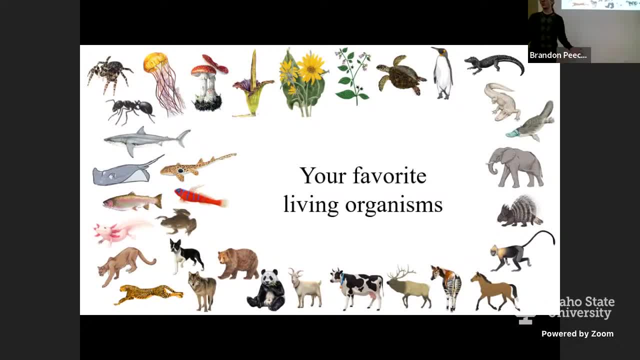 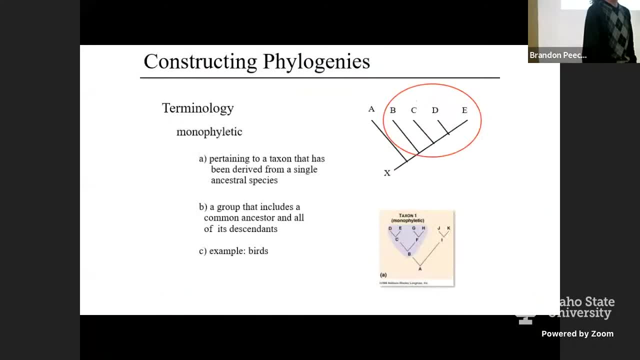 We'll go alligator mushroom and then flower. You guys will be like: but it's real, It's true. That is clade and node and sister group. Those are the words I want to make sure we get. I want to hear about monophyletic groups now. 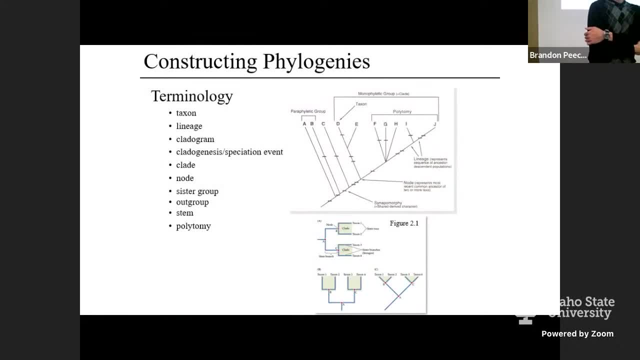 What is a monophyletic group? This is an important thing. I like that you guys have circled on both of these dry erase boards, so I'm not really worried about it. but can somebody put it into words? What makes a monophyletic group or a monophyletic taxon? 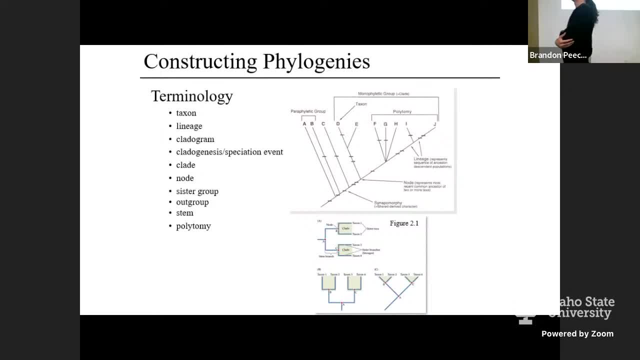 A taxon is for sure something that is usually the clade, the monophyletic clade, the taxon. How do you define a monophyletic group? Monophyletic group is any clade that includes all of the ancestors. 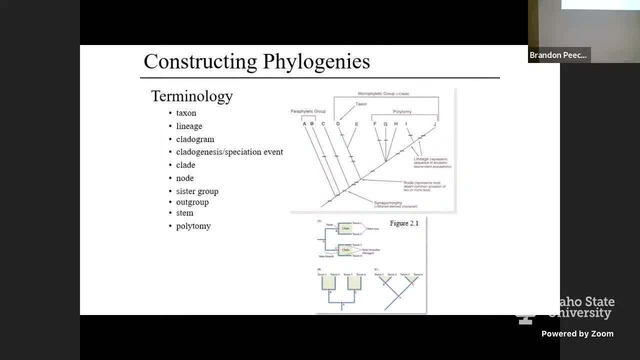 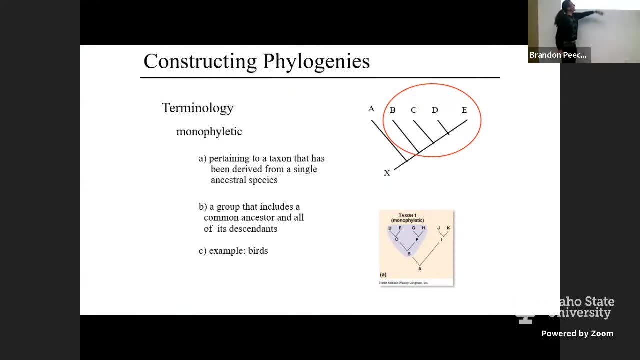 All of the ancestors, all of the. The simplest definition I want you guys to burn into your brains for monophyletic group is B. right here It's a common ancestor in every single thing that comes after that. common ancestor On this phylogeny here of A, B, C, D, E. 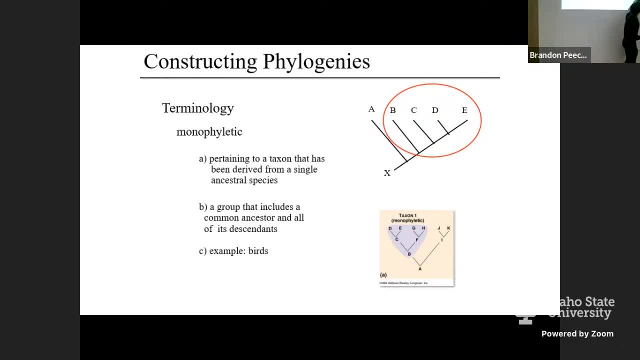 the common ancestor of B, C, D and E is down there. If you are including that in your definition, that right there in that red circle, whatever that thing really is, we would call that a monophyletic Group. Here's these two organisms here. 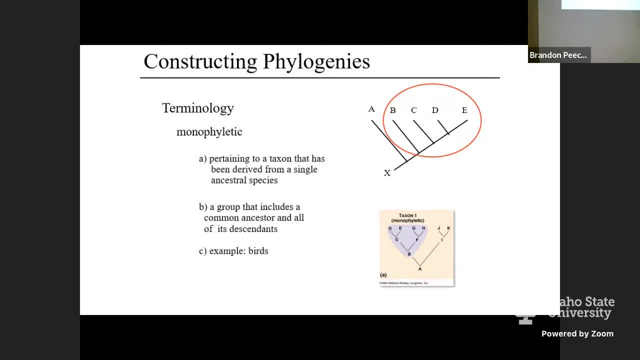 They both have their own lineage. They have a common ancestor. If you have a clade whose name means everything, this common ancestor and all of its descendants. so in this and this, that is a clade: the great taxon. I bet you guys know what this clade is called. 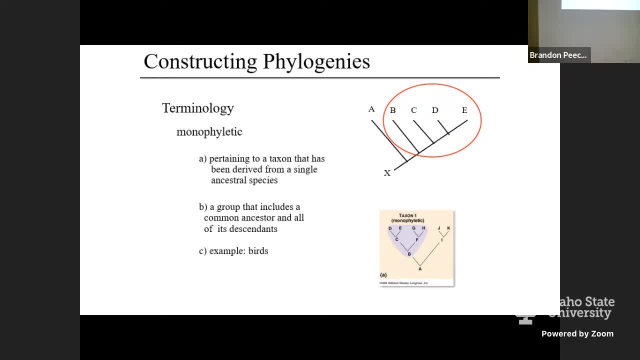 On this tree. what clade is that Plants A blood? No worries, You can get really specific and tell me the actual, sub-ordinal level of things that are between, specifically, a nightshade and a corksflower, because somebody like nightshade. 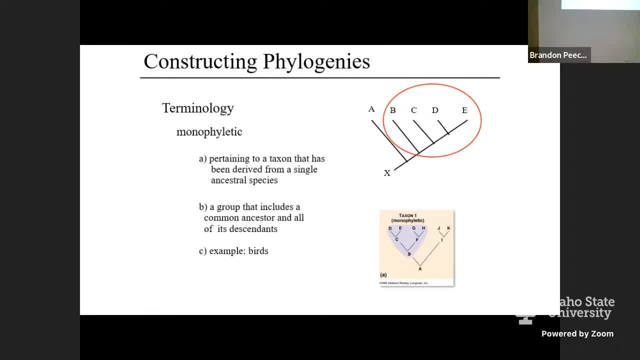 they'll be like a corksflower. But I could also say on this tree: that's just plants. and I do it again: That is just plants. That's a monophyletic group, a common ancestor and all of its descendants. 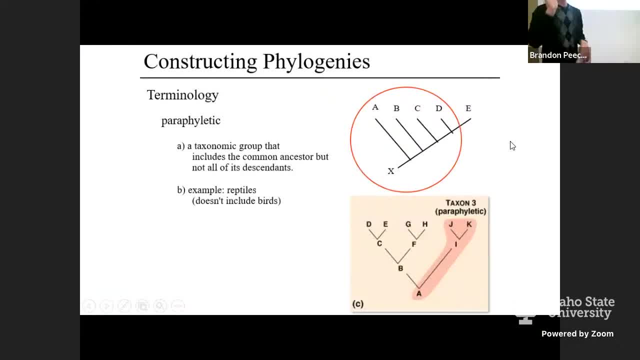 I don't know why that's happening. The only reason we talk about this is because very often in biology there are good reasons that people have named groups of organisms that are paraphyletic. I won't have you guys define this really, but you can see on this example here: 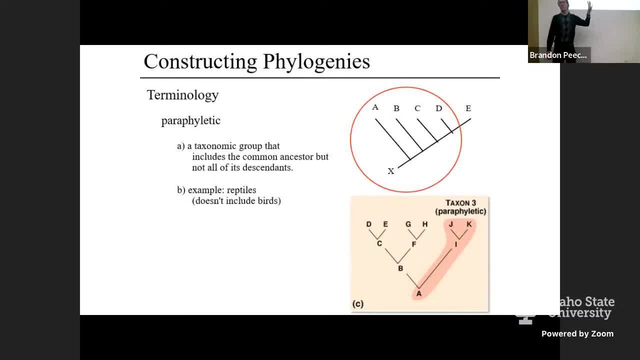 If you had that common ancestor but not everything that descends from it and you call that a thing that's a paraphyletic group. It's not great for evolution because it makes evolutionary studies, but it might have functional utility. A great example that we already talked about in this class is reptiles. 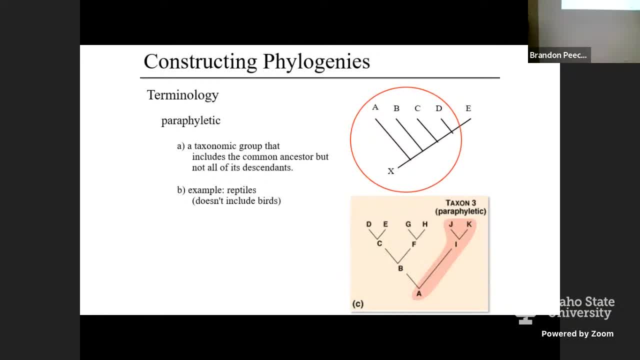 You guys might think the turtle and alligator should go together for totally great reasons. They're scaly, they're ectothermic, they're in the tropics. that's fine If you were to circle the turtle and the alligator, but not the penguin. 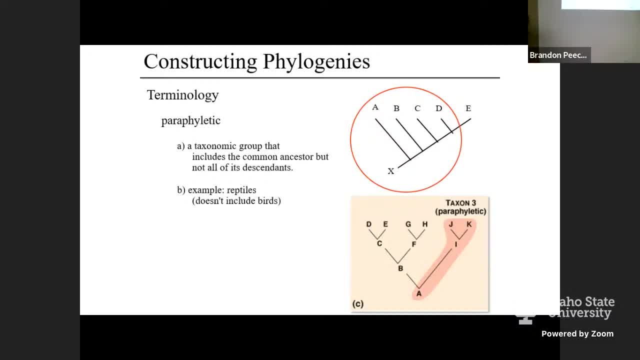 The penguin is feathered and warm-blooded and all those other things You're saying. the alligator and the turtle go together in some ways, but that doesn't reflect their evolutionary relationships. You can say that they're reptiles, lowercase r. 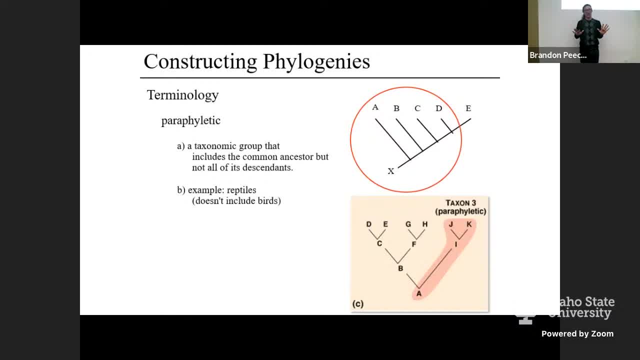 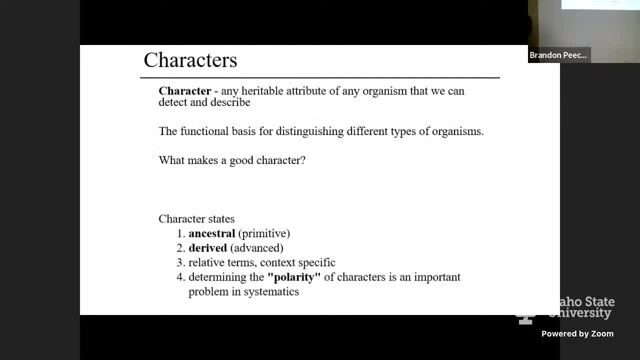 That's a paraphyletic group. Biologists, we're going to pull away from that because we care more about relationships and what that shows us. If we put reptiles as turtles and alligators and lizards, but not birds, we are robbing ourselves of. 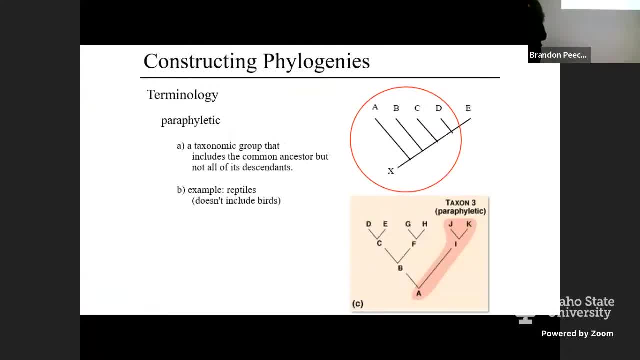 understanding something about the real biology of these organisms. Alligators have a ton more in common with penguins than you might expect, so we would have to talk about that. That's just something I want you to know. The simple thing is that monophyletic group 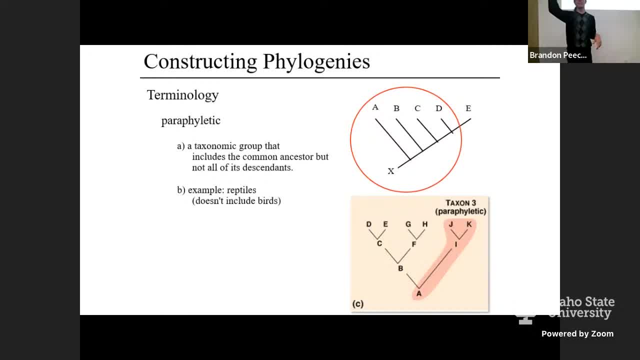 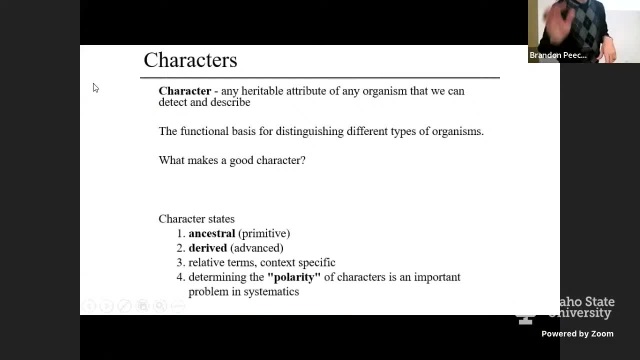 common ancestor, all descendants, paraphyletic group with a common ancestor, but not everybody. That makes sense. All of the phylogenies you're ever going to see, even if I just whip one out, I just threw this one up here. 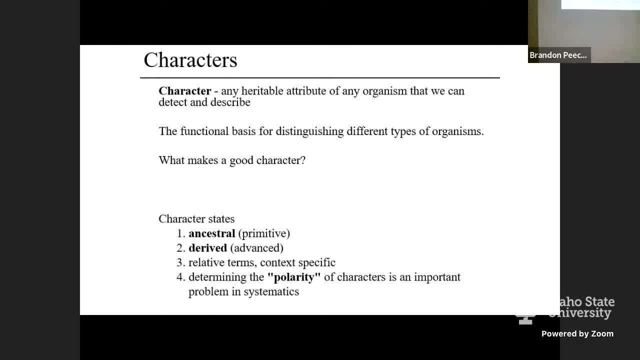 are going to be based on evidence. That evidence could be genomic, it could be all kinds of things. In this class we're going to be focused a lot on comparative morphology, anatomy- Anything that is used to inform a scientist, to make a phylogeny. 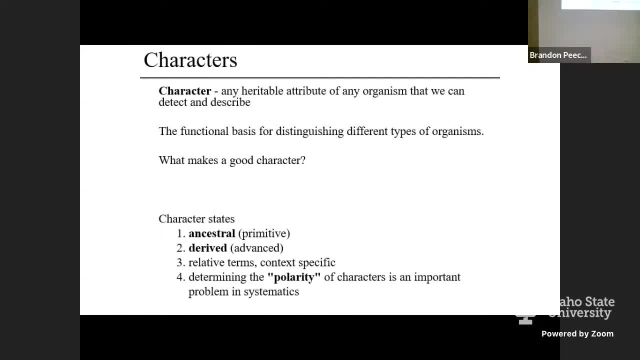 can be called a character. It's like a feature, it's a trait. A character is something like this: Now you want it to be heritable, You want it to be something that evolution works with. It's how we can tell different things apart. 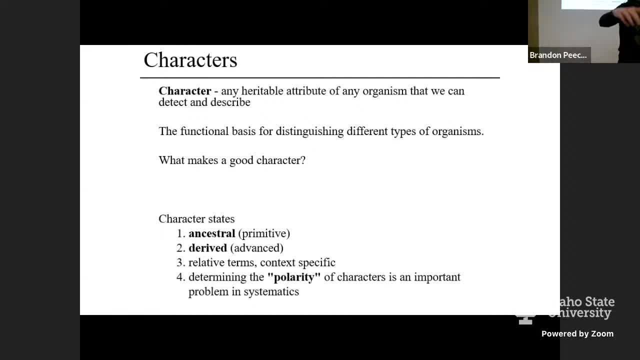 This was another thing on your worksheet. Can you talk in your bigger groups of seven? what would make a really good character something that is valuable for us to determine the relationships of organisms? What features might define a good character? Are you going to get some volunteers? 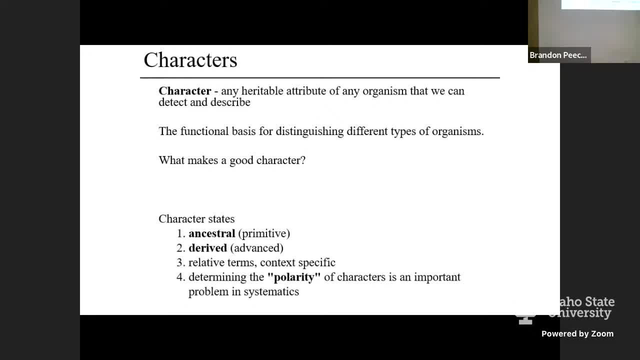 which group from the groups. just to give us a couple of ideas. what makes a good character? Yeah, Kevin, Distinctive, Distinctive. Yeah, like a heart. Do you think there's a place on the tree of life where heart? 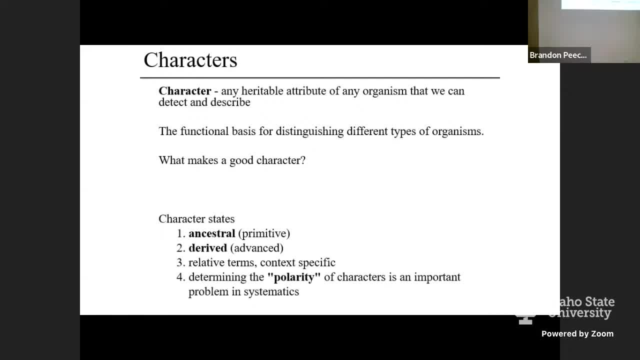 no heart is a good character. At some point hearts have to evolve, because not everything has a heart. Somewhere in the tree of life, heart may be a good character, But after that, if you're comparing all the monkeys in the Amazon, 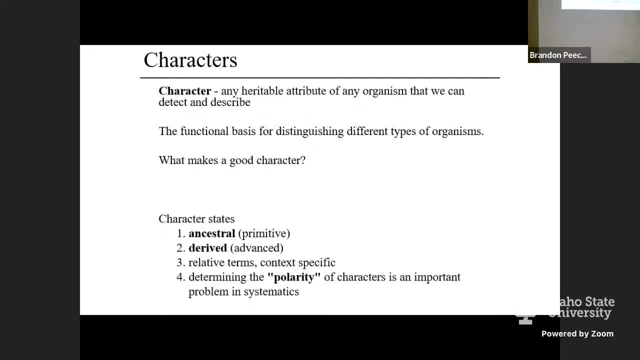 you're like heart- guess what, They all have a heart. not that helpful, But it's something you could detect. What else, What other things can make a good character? We just had a couple of general terms. Yeah, go ahead. 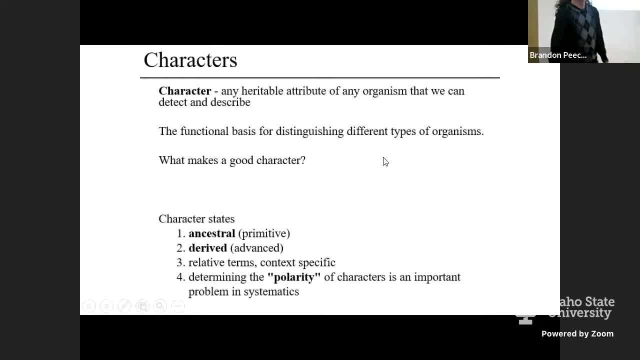 You said it needs to be observable, It needs to be consistent across the population. Okay, It needs to be measurable. It's a measurable. this is the population. like that, I think this is a great one. So this is an example of like. 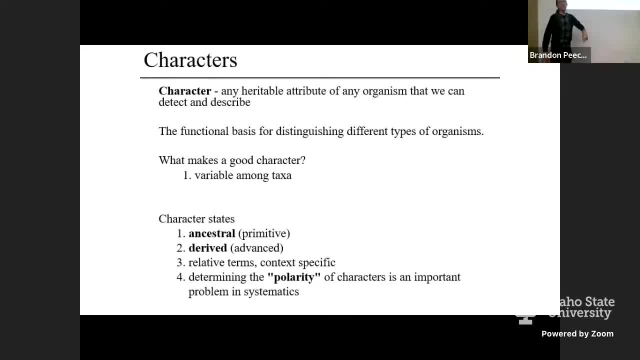 I like everything I just heard. by the way, Variable among taxa means something like when you are making a phylogeny. I hope you have some focus in mind. You're not doing all of like. I don't want to be a hunter with all at once. 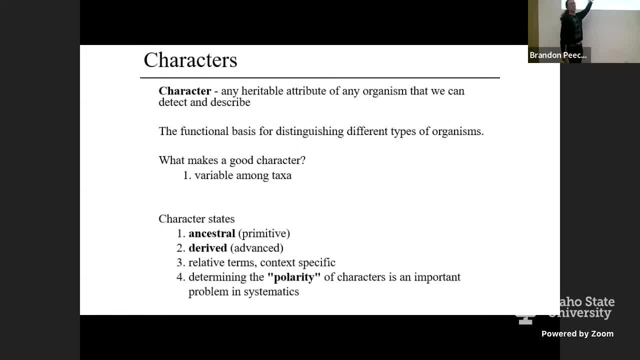 And so if you're doing South American monkeys, variable among taxa, heart wouldn't be a good one, but something else that might be a good one. So you want to be cognizant of what you're trying to get at and how it's variable amongst your study organisms. 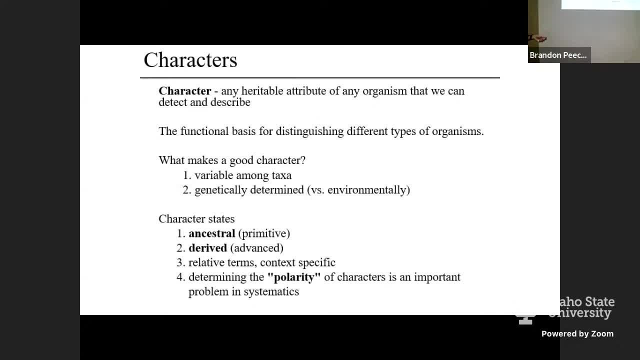 That's a really good thing. This is a big one And I heard you guys kind of talking about this before I asked you Genetically determined, something that's like heritable. So there's tons of examples in the natural world where, like if you're a plant in the desert, 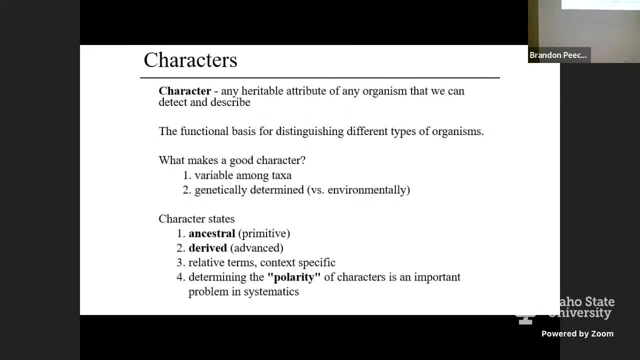 versus a plant in the rainforest. you're the exact same species, but you might have smaller leaves or grow shorter. That's an environmental plastic response to habitat. That's not something that's genetically determined And it might give you false results. 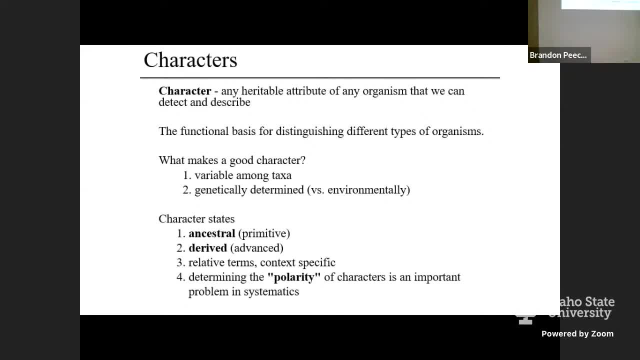 You put this plant. that's the same species, but some of them are in forest and some of them are in the desert. They don't look like each other. So genetically determined is a good one. Whoops, There is another thing, isn't there? 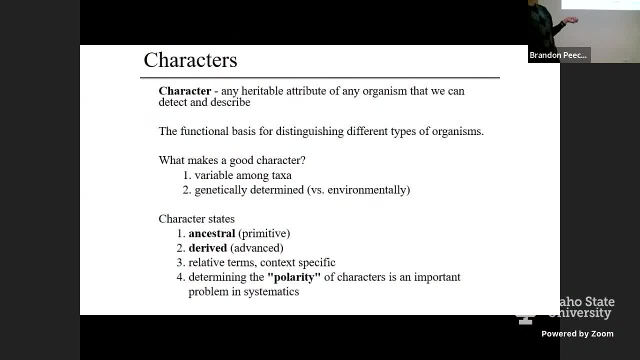 All right. Well, I don't know what's going on with my slides. They're like automatically advancing and there is a number three, So I'll figure that out. I wanted to ask if you guys could throw any characters up here. Some people already have. 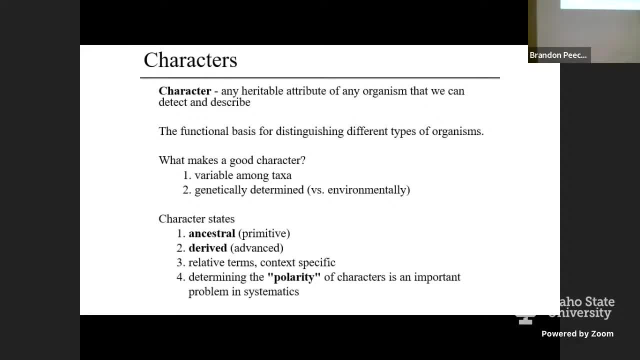 because they're being painted. So, indeed, yes, Chloroplast is a great character, And if I were to put a mark on this tree to say where Chloroplast evolved, well, this thing has Chloroplast, this thing has Chloroplast- I could say that they each independently. 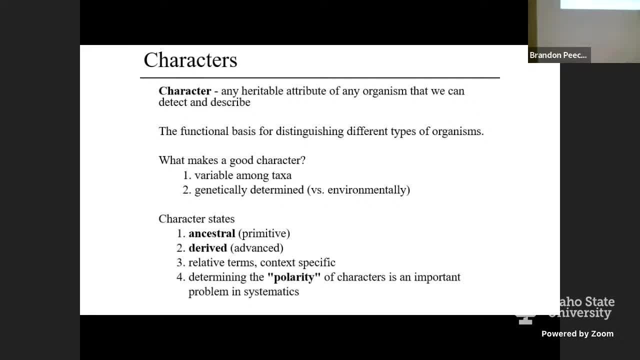 evolved to Chloroplast, or I could say that they have all. the common ancestor had them and they both inherited them. Any other characters you guys would throw up on the stream? Are you comfortable with it? Yes, There it is. Oh, look at this. 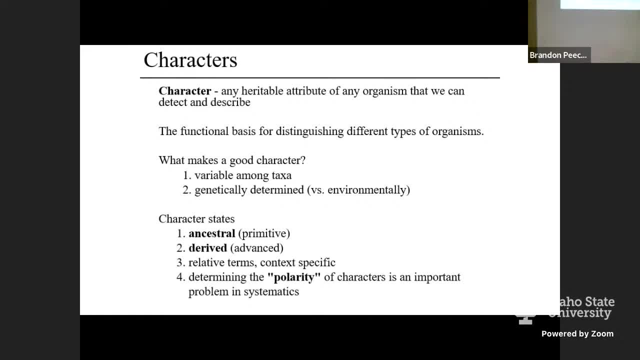 Mitochondria. This is a great example of an evolutionary hypothesis we could test. Did that mushroom and that nightshade and that cheetah all inherit mitochondria from their common ancestor, or could they each independently evolve it? or maybe two of them just evolved it? 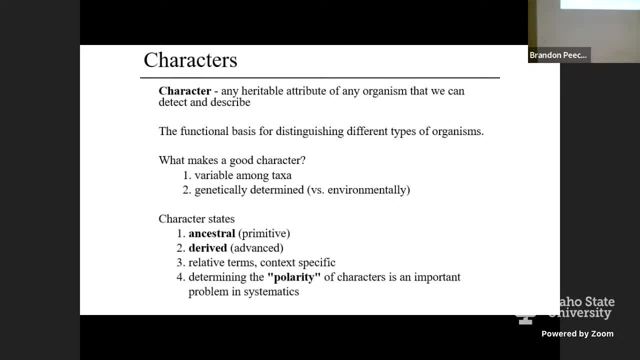 We could test that. That's a great idea. What's another character we could put up here? It looks like a skull shape. Where, What do you mean? Like diapsis versus synapsis? Oh, can you say more what that means? 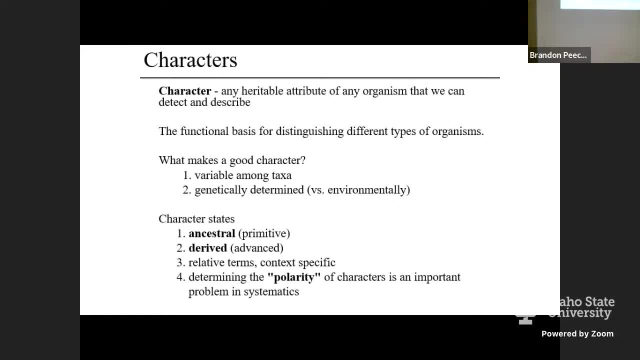 I don't know if it's going to be diapsis or synapsis. Yeah, the turbals. Yeah, So he's talking about the muscles in the temporal region of the skull. So mammals only have one hole. You guys have one hole. 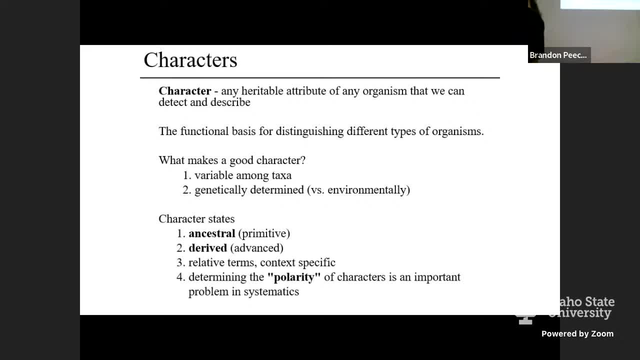 We'll talk about it later- And all reptiles ancestrally. it's kind of a mess, but have two, And so there's a split here: two holes, one hole in the skull. OK, So we have two holes in the skull or jaw muscles. 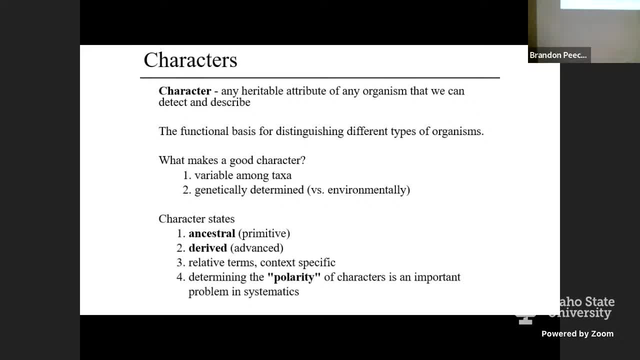 Doesn't it make you- and I hope the answer is yes, doesn't it make you go a little bit bananas to be like: well, wait a minute, what's the deal? Anyway, that's way too doomed in on what my lab actually does. 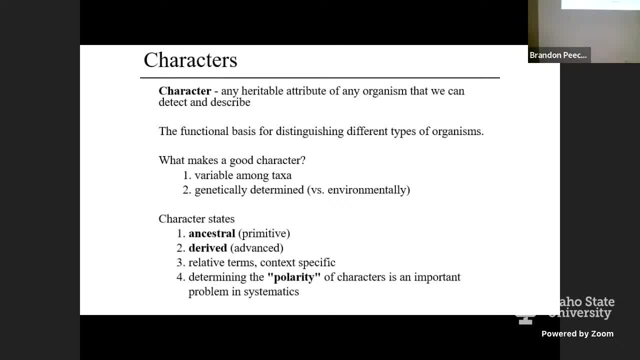 What's another thing? I mean, some of these are up here, right, Fur milk. Do we agree with fur and milk going here? OK, so what is this? Could be mammals, I'm going to say placental mammals. 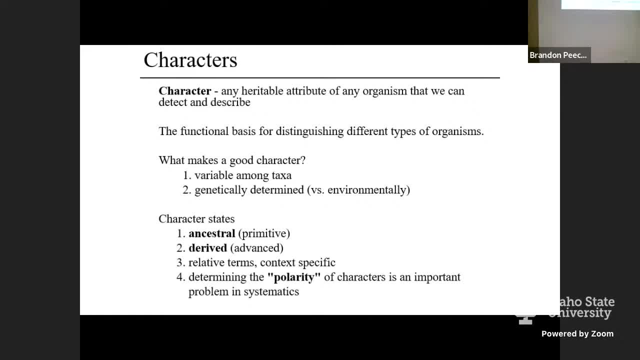 but they're the ones that are the ones that are the most important to us. Yeah, that's great. So I just hope you guys can see we can make this go crazy. So this is like dogs, bears. You don't know what this is, but I'm going to write it. 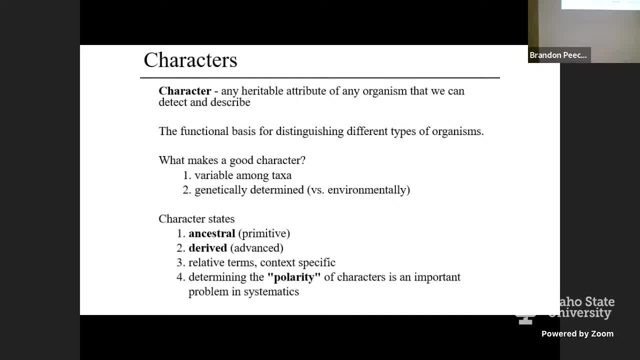 Caniforms, carnivores- We can go back and back, and back and back. Oh, this is a great one. Eurasia bears. All of these things have names, And so we can go. you know this one, I bet. 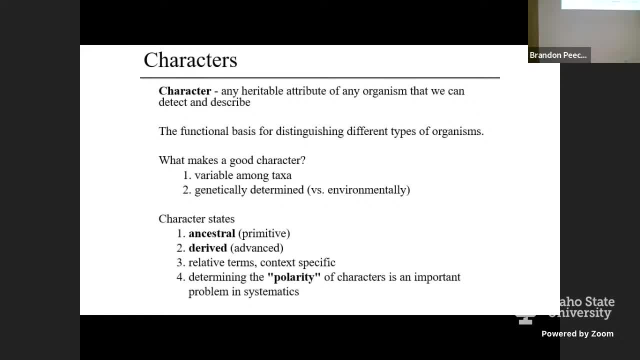 Thank you very much. There are actually these things that almost are really sisters- the cats- so i can give you a really specific name. anyway, just an example. there we're going to talk about character states and how they help us understand evolution. what's important about them. 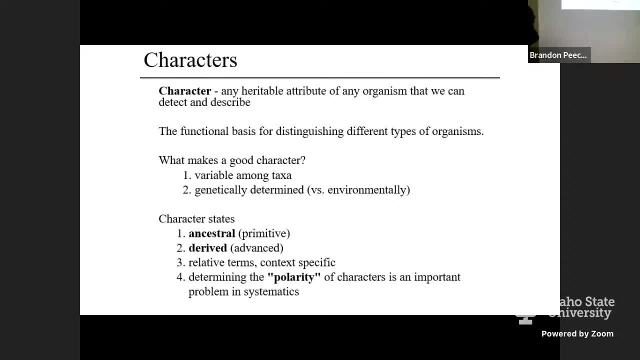 is that a character is like a statement. so fur is on here, but the character would be like presence of fur, presence of hair, and then the character state would have when we scored, when we looked at all the organisms we cared about and measured the thing we're talking about, we would score them. 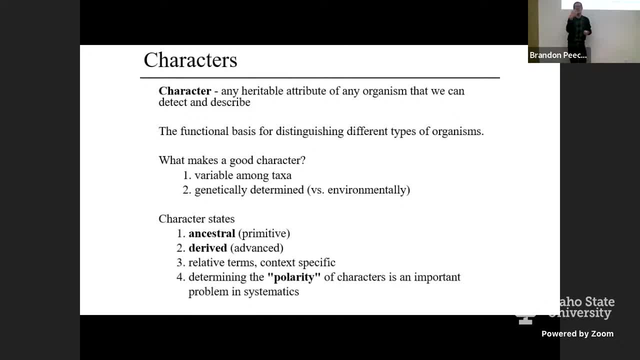 and some of them will be scored as ancestral or primitive. we're making another hypothesis here, and some of them will be scored as derived the advanced character. these words are outdated, a little bit unpleasant to say. it makes evolution seem very linear. it's not so. these are the words. 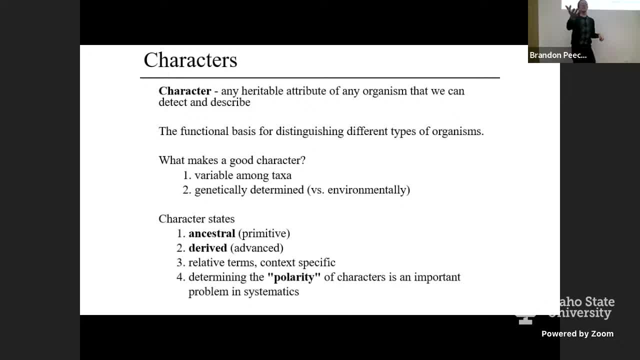 we'll be using ancestral and derived, and so we might say: i bet mammals have fur. mammals only have fur. so when i take all these amniotes, i think that the ancestral condition is no fur and the derived condition is fur. and so because it's a derived thing, 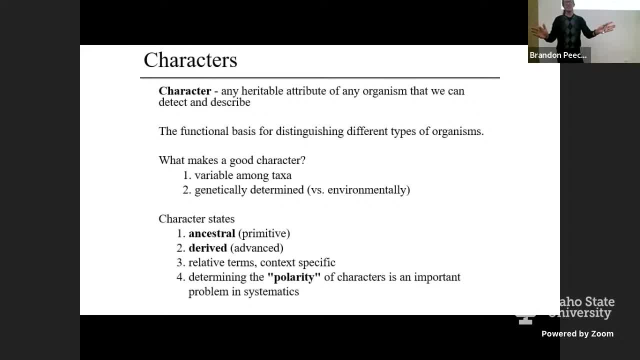 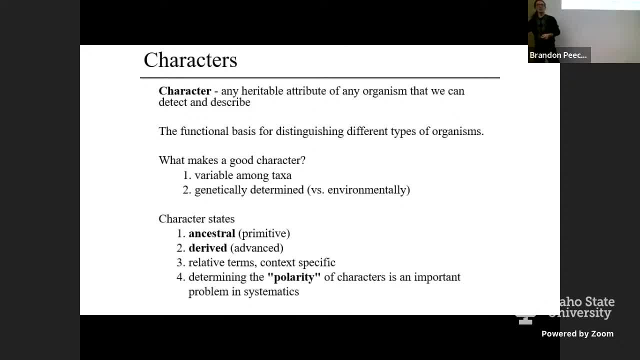 calvin's example of a heart way early back in animal evolution. a heart is a derived characteristic and other animals don't have it. but once you get up into monkeys, all those monkeys ancestrally have a heart and it's not interesting to talk about the presence of a heart. there might be details. 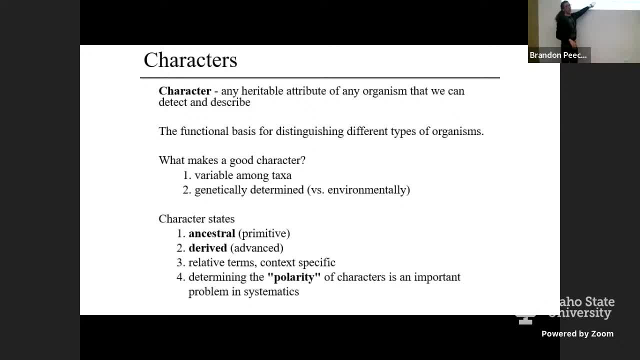 in the heart that are interesting. so these are relative terms. we're gonna have a lot of sliding around. and then there's polarity, because it helps us understand evolutionary transformations, so what is ancestral and what is derived and when that change happened. did fur happen here from a no fur to a fur lineage, or did? 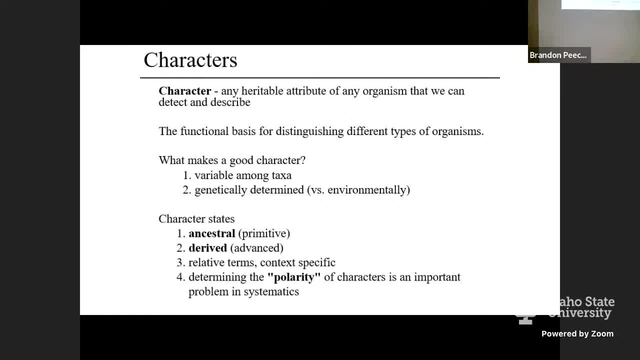 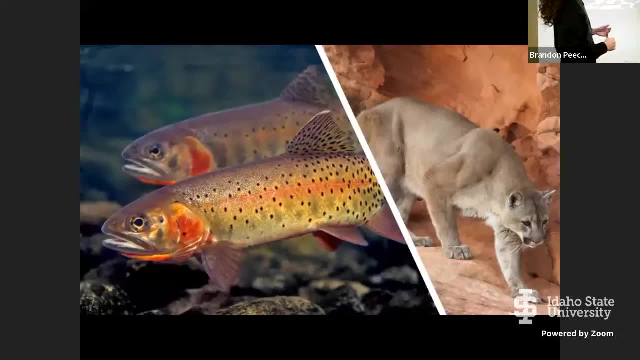 it happen here, and these guys just compared to their fur, and then these ones lost their fur. i don't know, but we can test those kind of ideas. okay, enough of me blabbing. here's two idaho animals. you don't know them, it's trout and a mountain lion. these are very observable. they're probably. 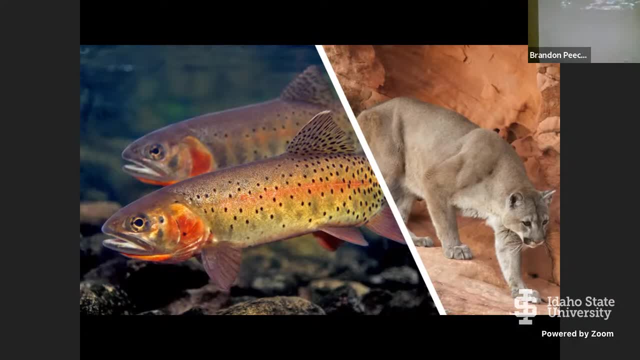 familiar to you. some of you probably can see what's inside of them because you know something about cats or you know something about- it's okay if you don't, but we're going to use these two idaho animals to make a big, big, big, i hope- list of characters and i want you guys to make hypotheses. 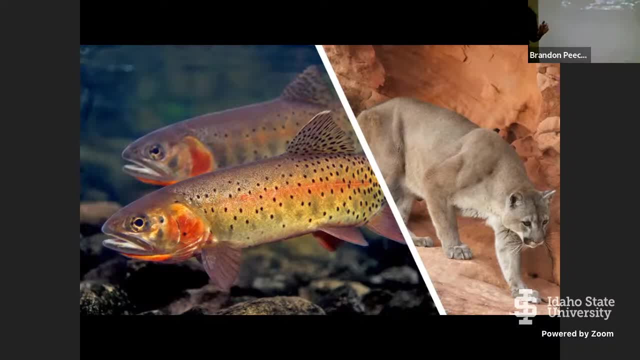 about the characters you're observing. what if the characters you're observing are unique to the mountain lion, are unique to the trout? what are shared by them? because their common ancestors shared them what are shared by them, but they did it on their own. they each evolved it and they're 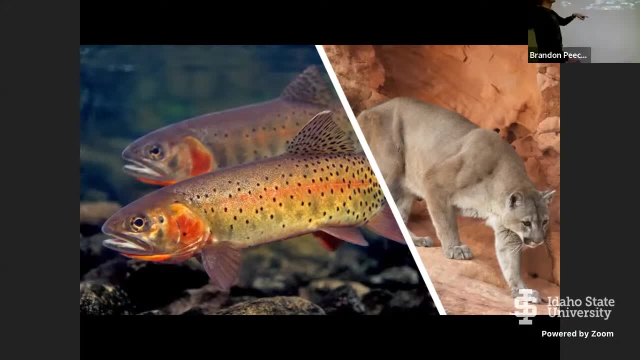 just happy to share it now. so these are very different things. i'll write this on the board. go ahead and chat with each other for a while. here you can be in your groups of i think your groups of seven is more fun for this. come up with a big list of characters that are unique to the mountain. 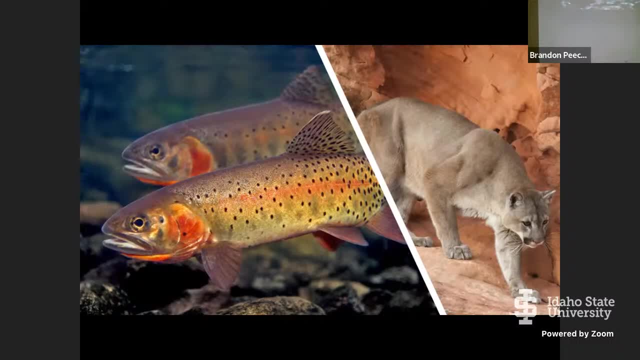 lion, unique to the trout, shared via their- i'm going to say- a, which is their common ancestor, which means the common ancestor of trout. mountain lions had this and they both have inherited from that common ancestor and versus shared and put that in quotes, but each of all the trade independently. 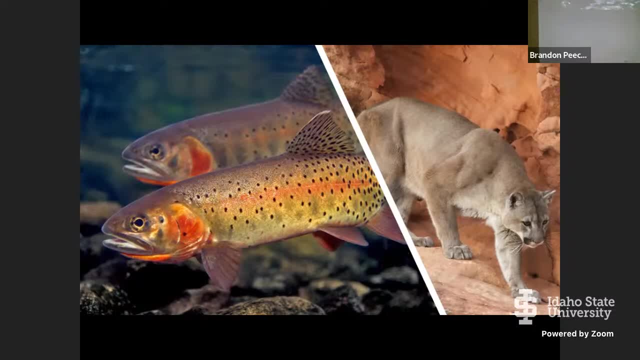 if this is all seeming a little bit wacky, that's okay. we'll get some examples going and then i think you'll get it. the shared driven is the same trade. it's what i'm not going to get to specific. it's something you can observe about them, okay. 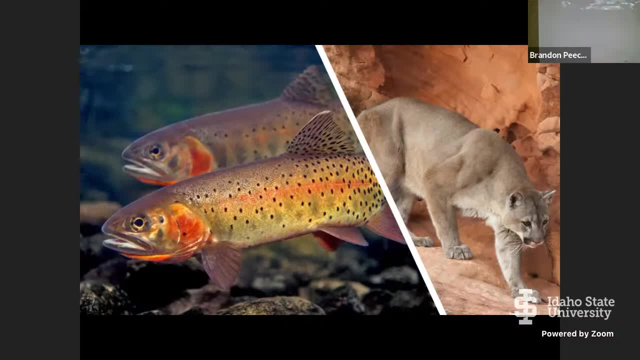 i've got this best for people like they're both brown, which is great. where do you put brown on here? which of those four categories? okay, or they will have brown. so go ahead and take a little minute here, talk about it. what features do you think anatomical? keep it anatomical. uh, you look. 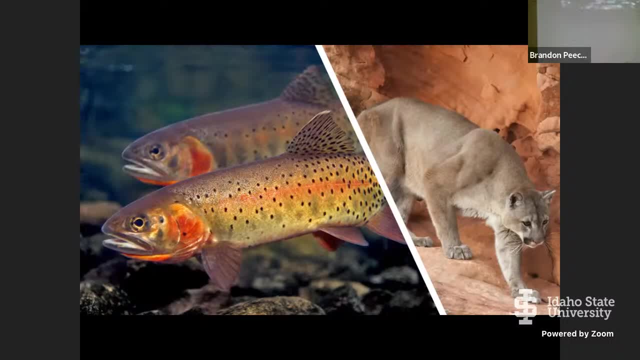 like i don't, don't do that. uh, keep it on their body plans, okay, so, unique to the mountain lion, unique to the trout, compared with both, because their common ancestor shared, because they will have it, but you think it probably evolved independently. and again, every single one of these. 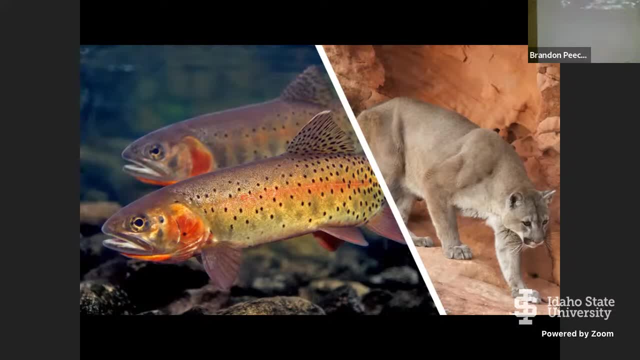 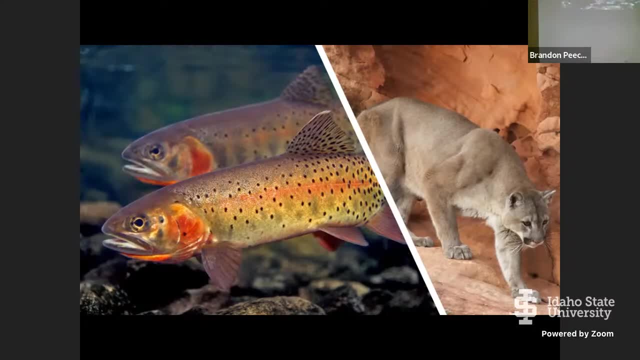 um, um, why? um, um, It was much stronger than all of it. Speak to us about it And you're on it, And you have the ability to. I mean we can just put the sensory work in The full time sensory work. 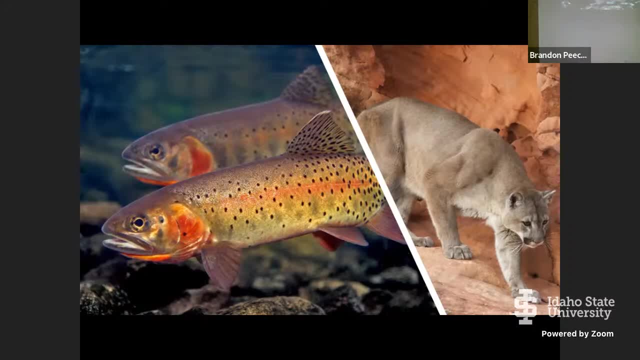 It's always about how to look at her, the whole thing and be proud of that. Technically, it's the best time to have an accessory, But what are the accessories? I guess I'm concerned about her. I don't think so. 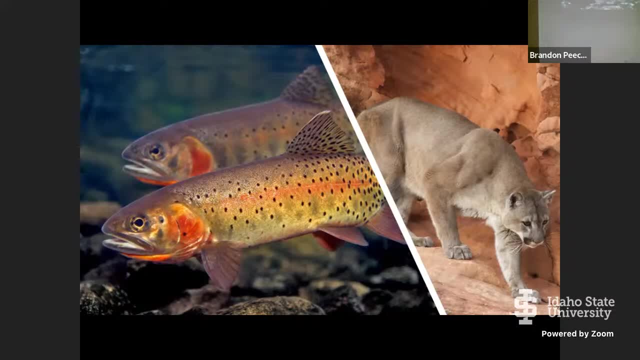 Yeah, I don't think so. Yeah, I have a lot of. I'm sure there's some. Yeah, I know, I'm sorry, I didn't, I'm sorry, I didn't, I'm sorry, I'm sorry. 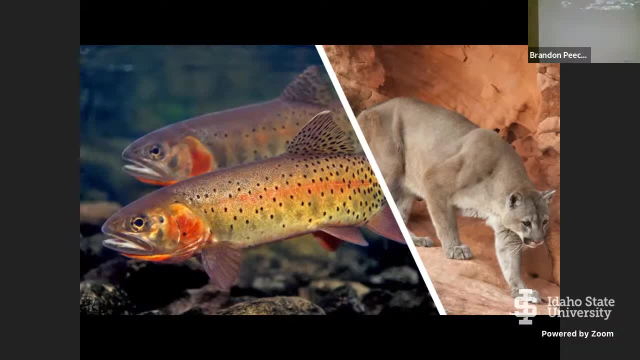 Oh, you know I'm sorry, I'm sorry, I'm sorry. Yeah, I know I'm sorry. all right, i'm just because i'm looking at the time i'm going to call you guys back. this is just an exercise and observation. i was hearing cool things, i like. i like, when i heard a little. 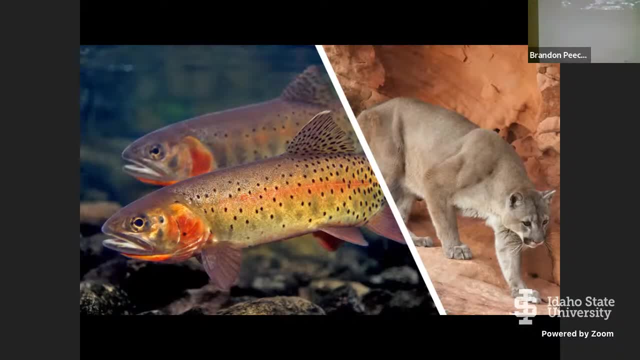 bit of a disagreement between you guys. that's great, forcing you, maybe, to be more specific. so, um, can i get some examples of observable characters that you would argue are unique to the mouth? you're just a pregnant dude, yeah, at least it's like fur cloth bones in their limbs. 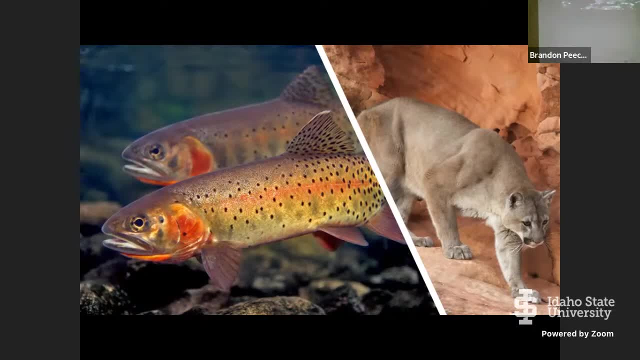 say it again: bones in their limbs. i'm gonna stick a pin in that one, because does the fish have live? so fun? we're gonna come back to that. absolutely, absolutely. these are arms and legs, but in a fish they never became arms and legs, so it's so wrong and inappropriate for me to call them arms and legs. but there's bones in those. 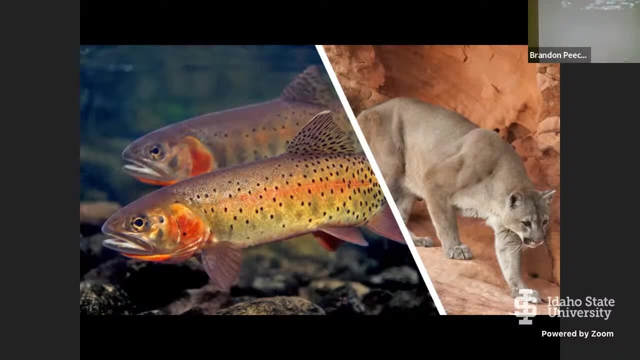 things, so i'm not gonna write that one down. what are some of them? on my own whiskers- whiskers, which is just fancy for her shoulders. what do we mean by shoulders? it's loose, right? you guys know something and we're gonna. this is what's so fun and why i 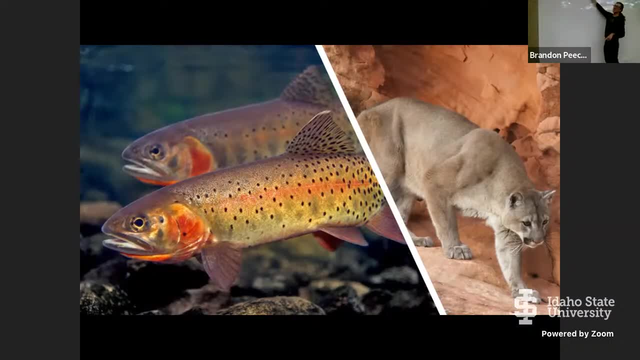 shouldn't do this. guys get distracted on every single one. there's one bone here in this thing and this fish's gill arch, there's one bone that is homologous. it's the same as your scapula, so there is a shoulder up in there, but it never, ever became. 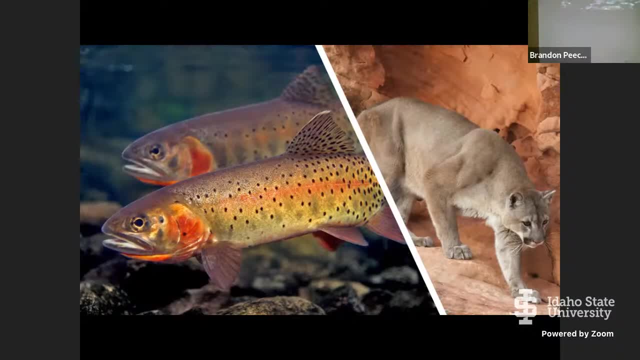 shoulder. i don't know what i'm saying, but i like it. i know what you mean because the functionality is very different. okay, what are some features you need to the travel? oh, these eggs, guilt, guilt, Fence, Fence, No, mountain lion with fence, What else Scales? 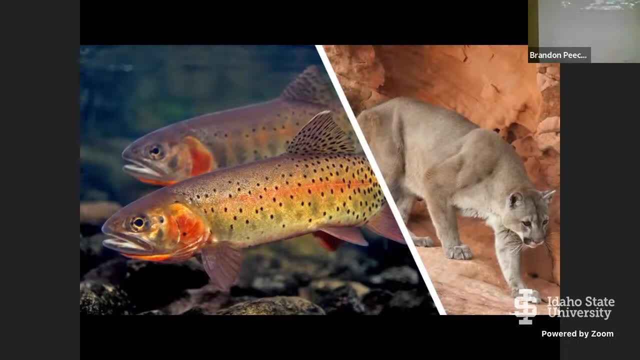 Scales. The lateral line, The lateral line- Awesome. I just want to say that these features are really excellent for determining how the trout are different from the mountain lion. Once we get more into this. some of these are all void. All right, What traits do you think they both share? 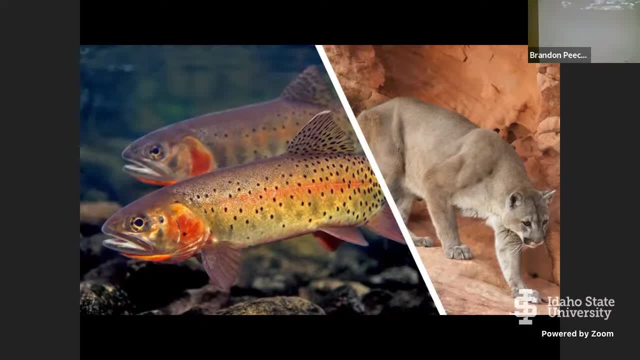 because the common ancestors of all fish and all mammals, bony fishes and all mammals shared That feature: Vertebrae, Vertebrae, The presence of a backbone, Teeth, Teeth. What else? A jaw, Eyes, Eyes. 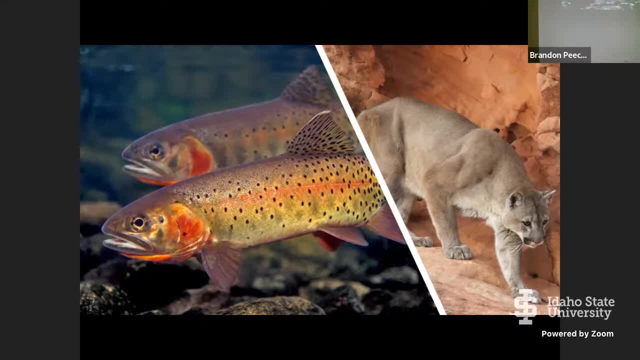 Then we understand that what we're saying here is: the common ancestor of mammals and bony fishes had an eyeball. Now they both have an eyeball today and that eyeball you can go through the lineages. That's really fun and really cool. 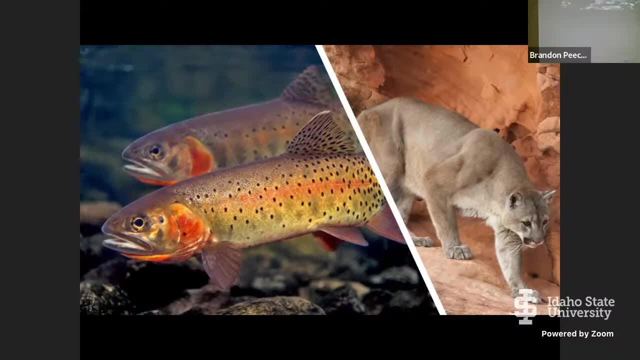 You might think maybe something else happened and then everyone's going to be like: what's the evidence for that? You get excited. These eyes are all against each other. maybe We're going to talk about that word in a second Vertebrae: teeth, jaws, eyes. 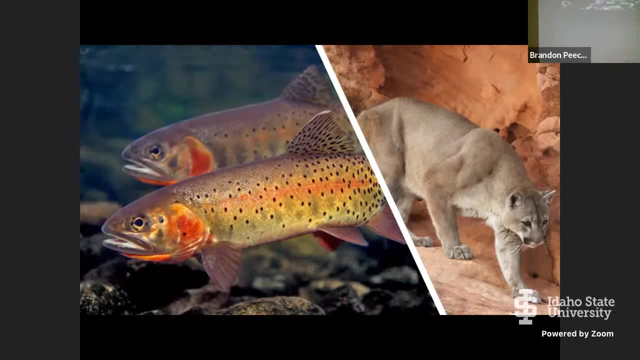 Any features you guys have that you think they share. they both did it on their own, not with their common ancestor. The fact that they're both part of the order- Oh, my goodness diet. I'm going to put a question mark by that one. 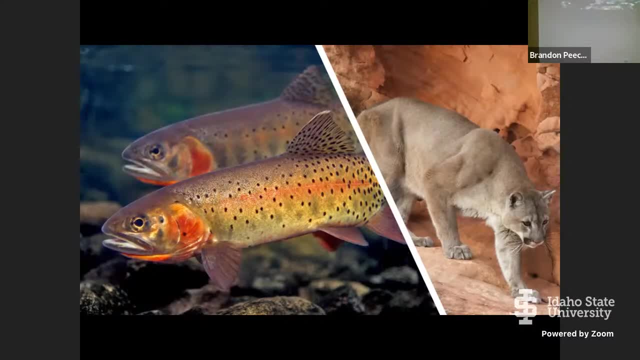 They are both carnivores, although I've found seeds and stuff inside the cow. What did you say? A tail? A tail, My goodness sakes, Is a tail a good example here, Interesting? What do you mean by a tail? 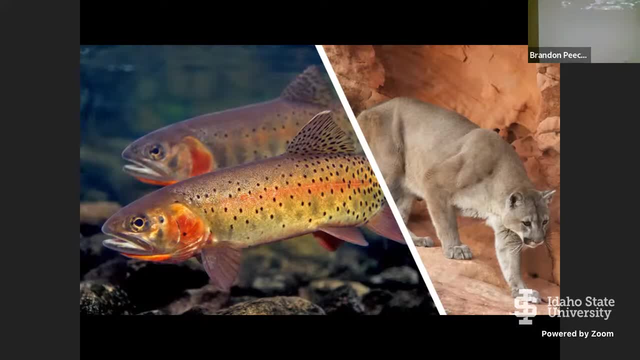 Actually, I'm going to go for it. I'm going to say that. What other things might they both have in common? Camouflage- They both are camouflaged in their environment. maybe If you thought that they both inherited environment-specific camouflage from their common ancestor. 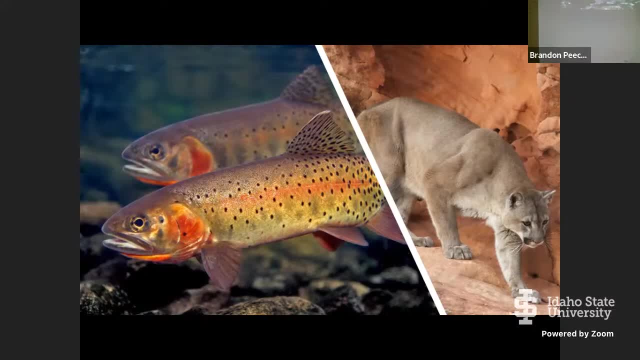 you might think that, But then what you're saying is that every single thing since the diversion between bony fish and mountain lions has had its camouflage to its environment. That seems a little bit independent to me. I bet you by the bet money. 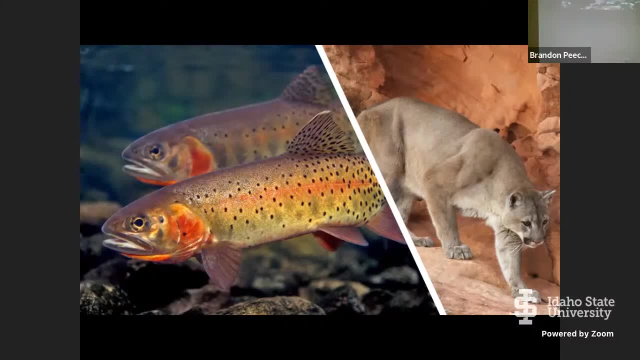 that their relative camouflage. they both independently evolved, probably pretty recently, when they are starting to live in the area that they live on. Also, I don't know about great camouflage. Mountain lions are just not really good at camouflage. Most of them are really good at being very still and intense. 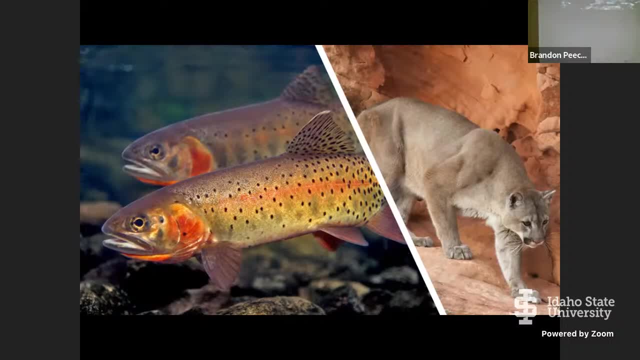 Because there's mountain lions in the rainforest and then mountain lions in the desert. They're both the same kind of color, But mostly just sneaky cat with the jacket. The point of this is we have, you guys, made some observations? I hope some of this is looking like. 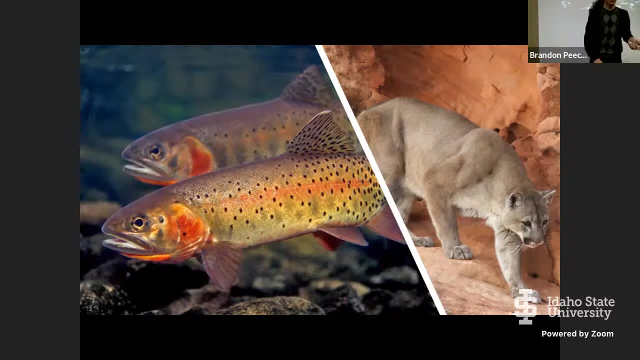 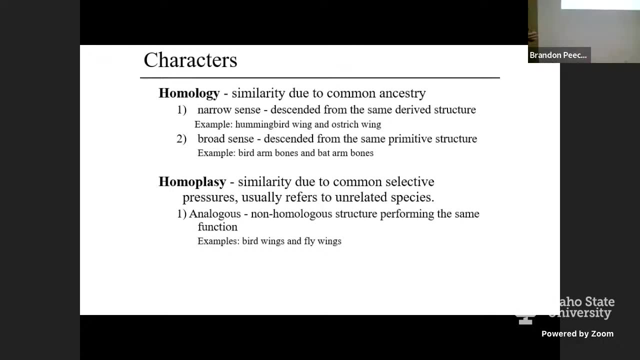 okay. there's things we can observe here. All of those are characters. all of those are observable. They're going to help us build a bunch of our words out. I used this word earlier. Homology is when there's a similarity in characters that's due to common ancestry. 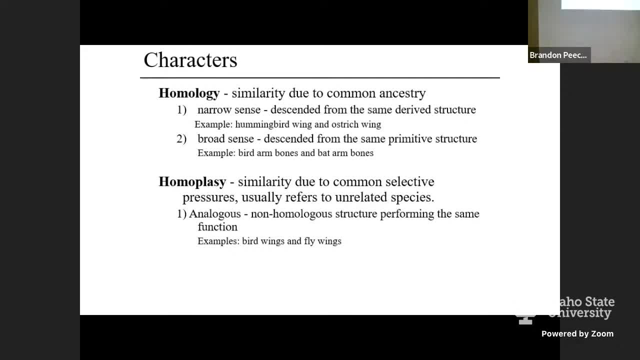 I will bet you everything I have: the vertebrate, teeth, eyes, jaws and the feet. This is very broad now because they're so different, but the presence of a tail, All of those things between those two organisms are absolutely homologous. 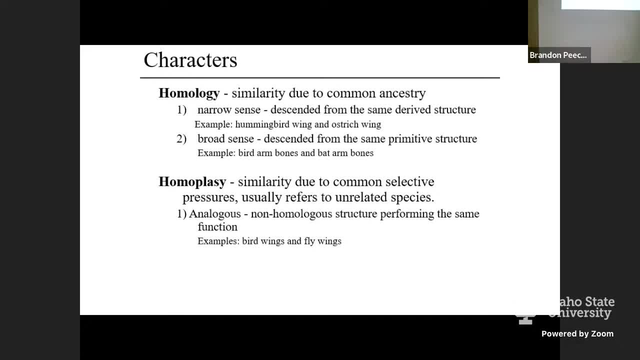 Your eyes, your teeth, your jaws are also homologous with that trout, just like with them online. There are a lot of different ways we could use homology. I put them up here: An ostrich and a hummingbird. both have wings that are homologous to each other. 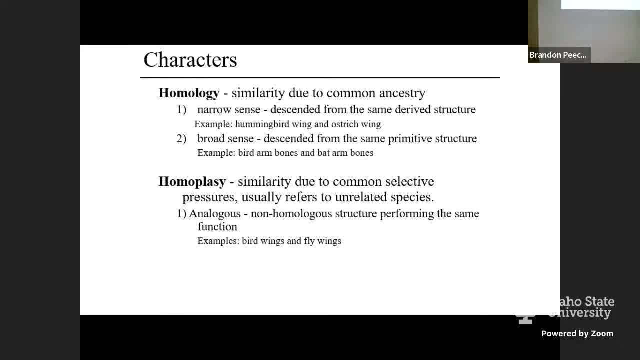 The hummingbird flaps it a million times. a second Ostrich does not fly. They're still homologous, But in a broad sense we can talk about homology too. Bats have a humerus and a radius and an ulna. 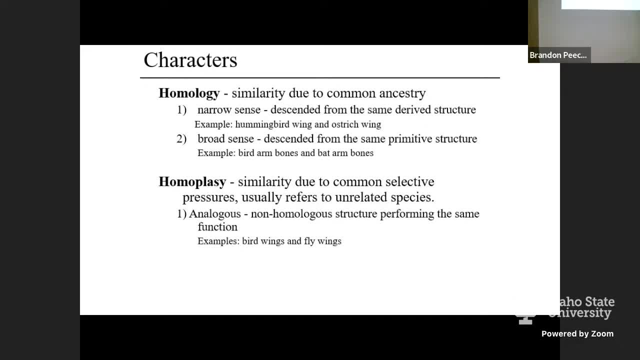 and birds have a humerus and a radius and an ulna. Those bones are homologous, but the wings of bats and birds are not homologous. One's made out of feathers, one's made out of skin, But the bones are indeed homologous. 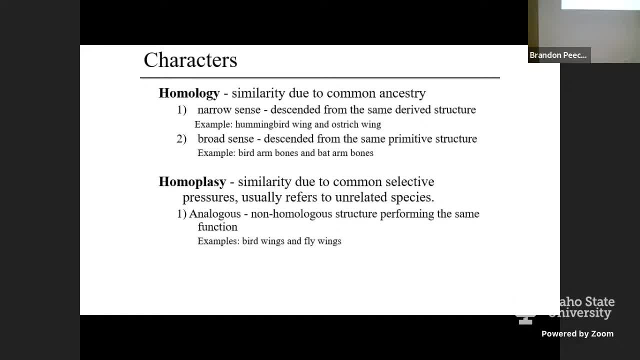 Something that's really important to this class, that we're going to talk about a lot, is homoplasy. Homo means the same, but homoplasy similar, but nothing to do with their ancestry. They didn't inherit that similarity from their common ancestor. 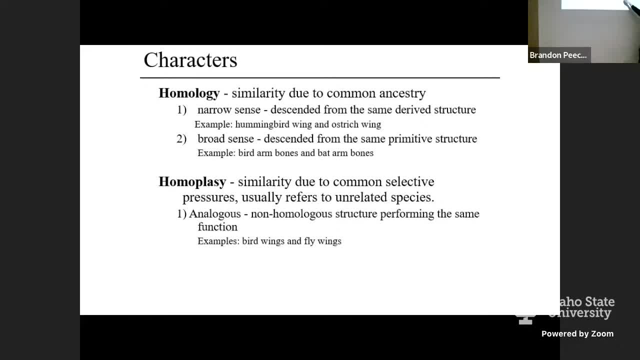 They're the same, but not because of evolution In a very broad, stupid sense. this is something from an intro textbook. a butterfly or a fly and a bird, both have wings. Those wings are homoplastic. But yes, check, they have wings. 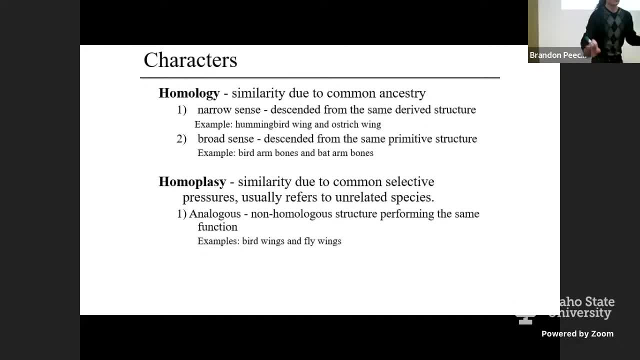 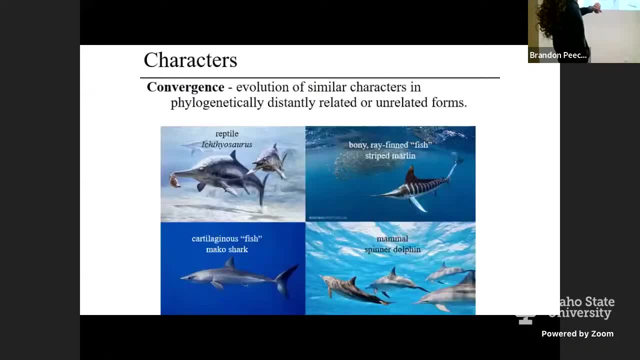 Those wings are not from the common ancestor of birds. They're from the common ancestor of birds and flies that independently evolved them. I think I'm going to skip that. We'll talk about that in a second. I'd rather spend the last bit of our class talking about this. 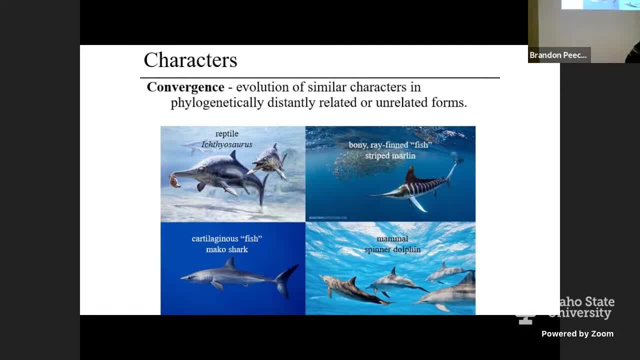 One really specific kind of homoplasy that I love and that Comparative Anatomy excels at teaching you guys about, is this thing called convergence. I know you all probably have heard of convergent evolution. Convergent evolution is a kind of homoplasy. 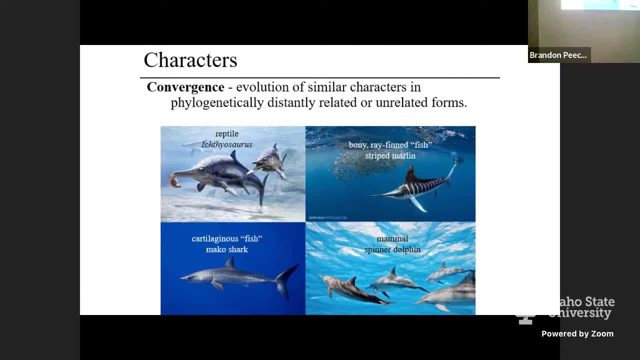 similar characters in, phylogenetically so on the tree, distantly related or even whatever it means to be unrelated things. I love this so much. This is a shark. This is a mammal. That is a bony fish. This is an extinct thing. 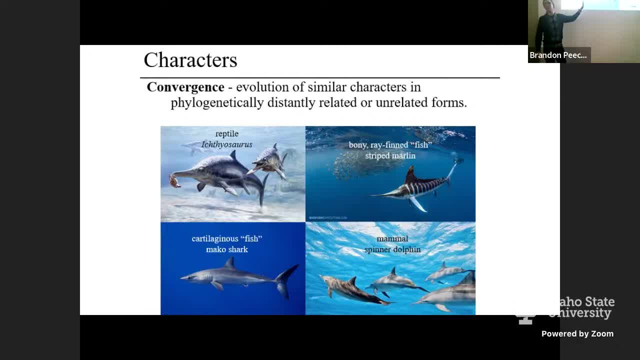 but it's a kind of reptile, That's all I'm going to say. A reptile, a shark, a bony fish and a mammal. Here's a picture of all of them. Please talk to each other, Make observations about these four completely different kinds of animals. 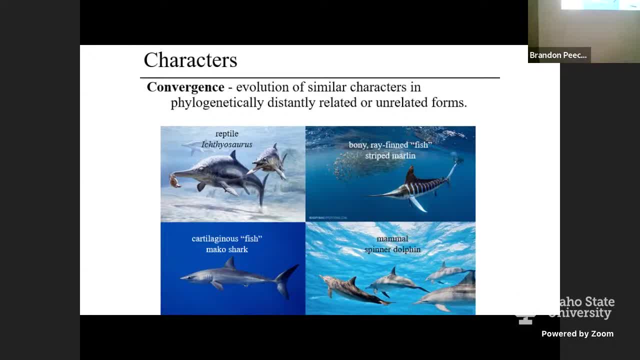 Go ahead. Okay, Finally, I wanted to focus on this. I think this will be like the beginning of this: Maybe this next section of this video where there's a lot of environmental knowledge in to know about mange and such. Probably remember that the above. 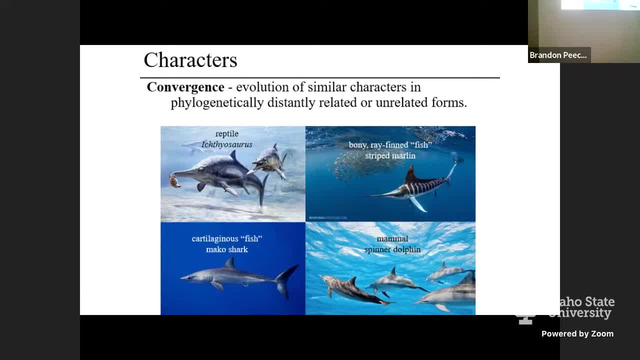 Well, if you didn't definitely like this, it's because I related to this video. I don't know if you're not familiar with OA-spirit to yoga, or yoga for me too. So, basically, you're not going to as much detail until you want to step into this. 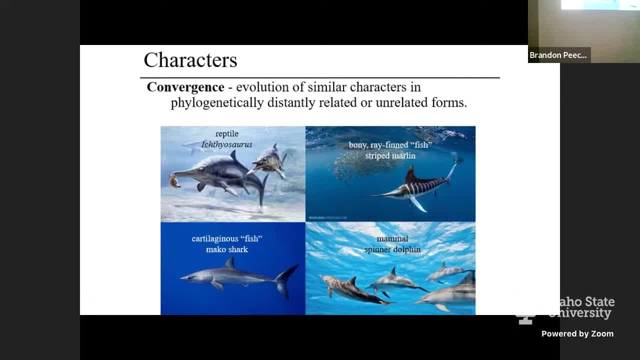 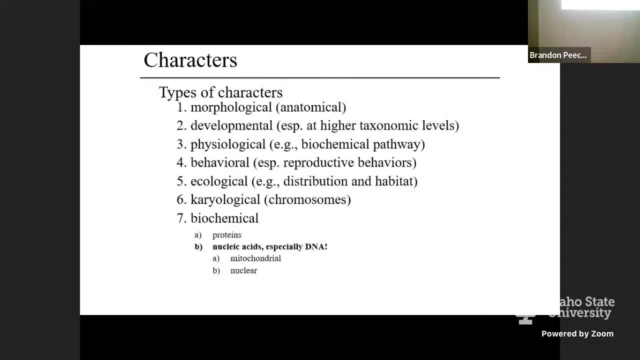 But what I really would I like to go to this day. I'm going to něe step over up here right now and we're going toemos that a little bit. Oh boy, I'm sorry, I don't know what's going on. 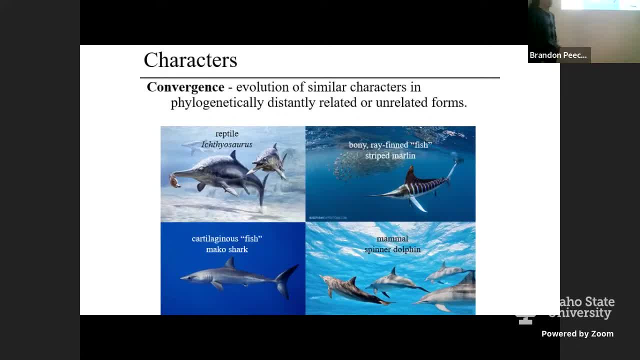 I don't know what's going on. Can I have some people just share out some observations they're making? Yes, Brian, Wow, Can anybody know what counter shading is? So you're dark on top, light on the bottom. It is a pattern you see again and again, and again. 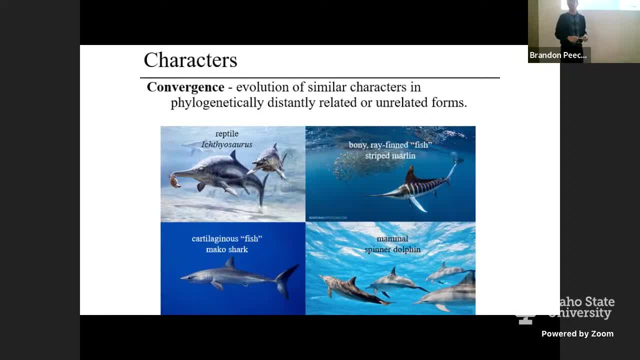 Out in the oceans. What is it? We'll talk about it later, But that is interesting, isn't it? Okay, what else Really streamlined body? Does anybody have any prior knowledge like what the ecology of these organisms are? I'm hearing marine, so that means the oceans. 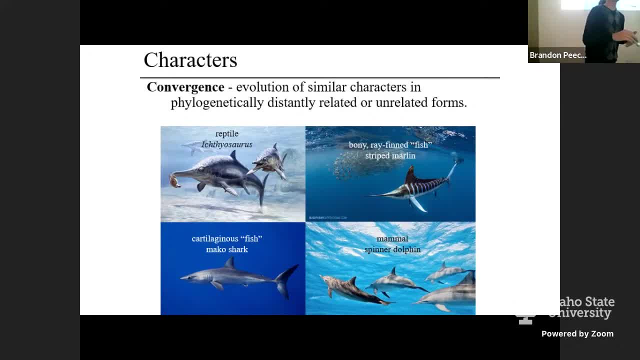 People usually say aquatic when they mean like rivers and lakes, and marine when they mean the ocean. So these are all marine organisms. Where do they live? in the ocean? I picked these pictures on purpose. Big open water, Yeah, What do they do out there? 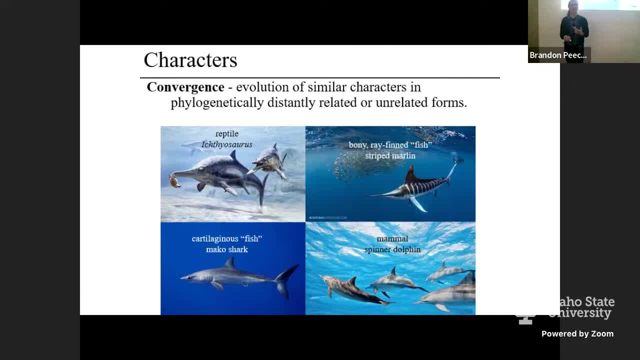 They're predators, and they're specifically predators of small fast things. None of these guys are chasing baby whales, like some sharks might be. This one is a fast eating fish eating squid eating fish eating squid. So they're open ocean pursuit predators. 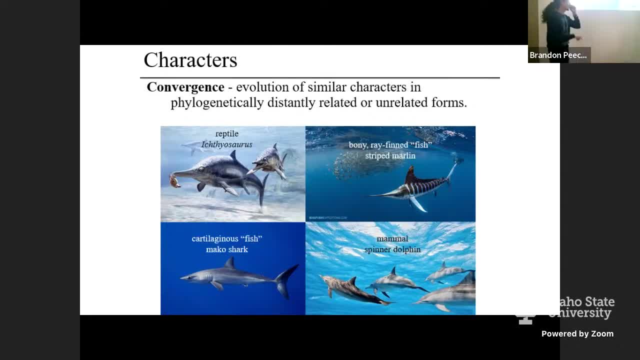 One's a mammal, one's a reptile, one's a bony fish, one's a cartilaginous fish. Okay, so you said strata. This is the first one, But it's a streamlining body shape. 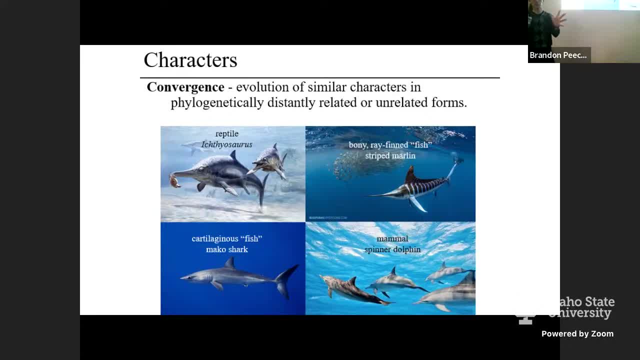 So maybe their niche space, the fact that that's what they do functionally, the fact that's where they get their food. evolution has pushed them all to be torpedoes, basically, which is crazy. What else? What other things? 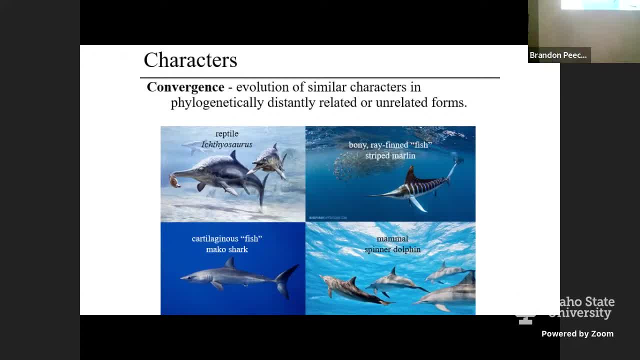 Dorsal fins. Talk to your neighbors. Tell me about homology or not of all these dorsal fins, What you think might be true. Go ahead and chat. I don't know. I'll try to talk a little bit, Okay. 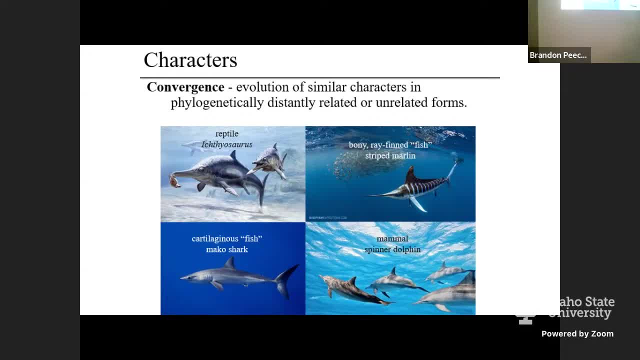 or one on top, This one, this is the one you see before the shark gets you all right. who has that? who has any? you can pick two. you don't have to do with the whole thing. any hypotheses about potential homology. you can start with observation. you're sitting there, you're aerosol, you're looking at the beach. 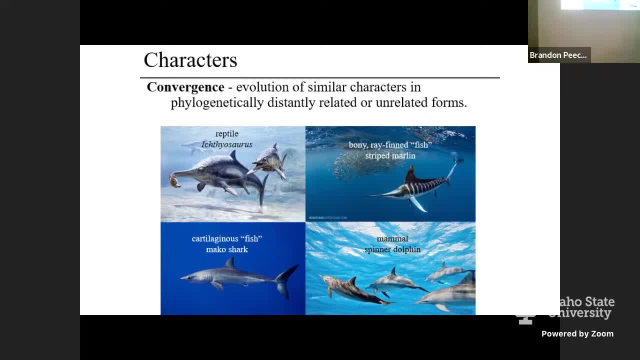 everybody's got a dorsal fin in front of me right now. homology of the dorsal fin. are they all homologous? they all inherit the same dorsal fin from common ancestor of all of them. if not, what else you might think is going on? sharks and the marlin would have homologous, because they never. 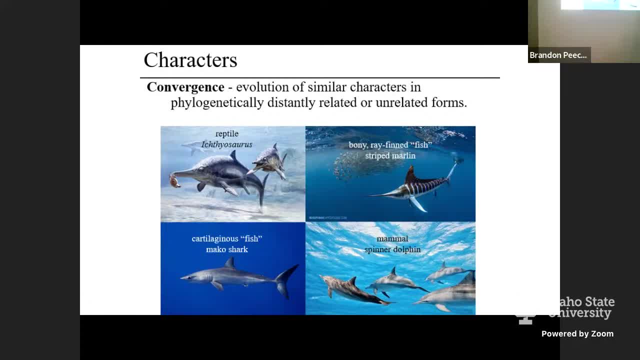 really lost them, they just changed. but the dolphins are the pathetic dinosaurs at some point lost. if you follow the dolphin, when you get back- not that far- you're basically going to be looking at like a little shrew thing. that's weird, but that's something we know. if you follow the 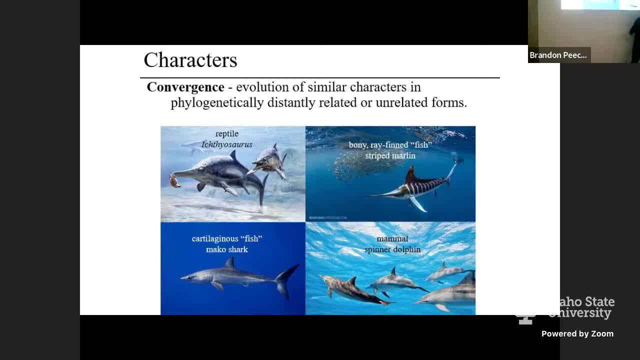 certainly needs back a little while it's going to look like a little lizard thing. these things have lineages that have never left the ocean, so the loss of a dorsal fin does characterize land animals like reptiles and mammals, and then both dolphin and igneosaurus have independently evolved- another kind of thing. 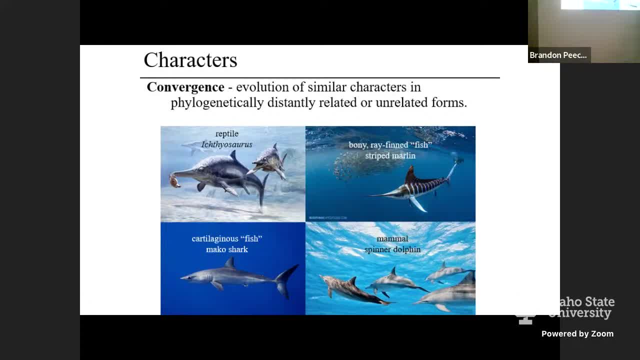 a dorsal fin. what is so crazy is there's obviously a reason for this. some of you were talking about what? what is the dorsal fin doing on all these animals? yeah, you're moving and it's like a little. you're a triangle if you look at it. in the front, they got these two fins and the one on top you can. 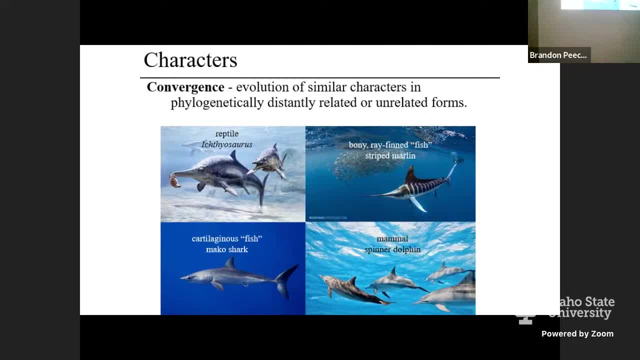 go through the water really quickly. it is absurd that a mammal and a reptile would have, like from selective pressure evolved dorsal fins and then look like this thing. this lineage has never, ever ever left the ocean. that's remarkable and that's why convergent evolution is so cool: similar environmental pressures resulting in similar